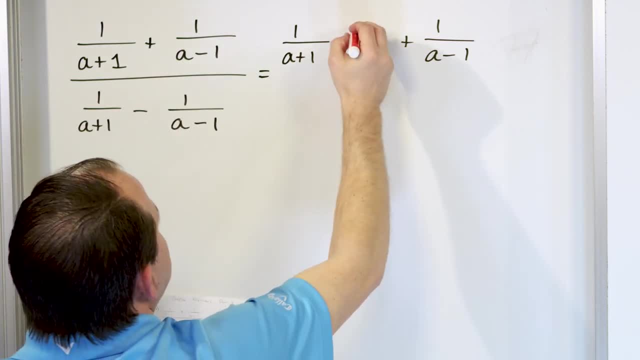 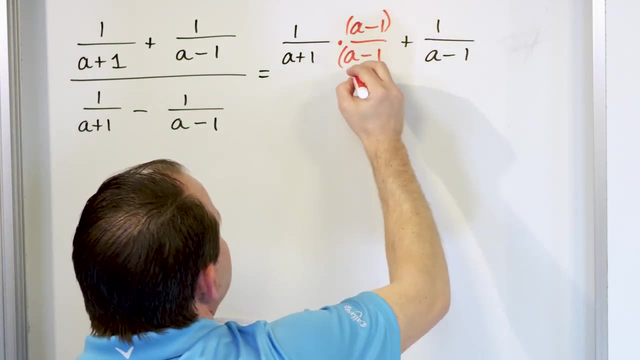 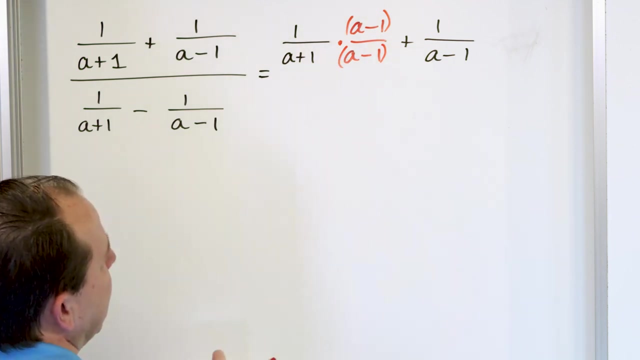 anything obvious. so I'm just going to take what's on the other denominator and multiply it by a minus 1 over a minus 1.. And if it helps you visualize, you can put little parentheses around these terms. So if I multiply this, the common denominator will be the large term, a plus 1 times a minus 1.. Okay, now to make. 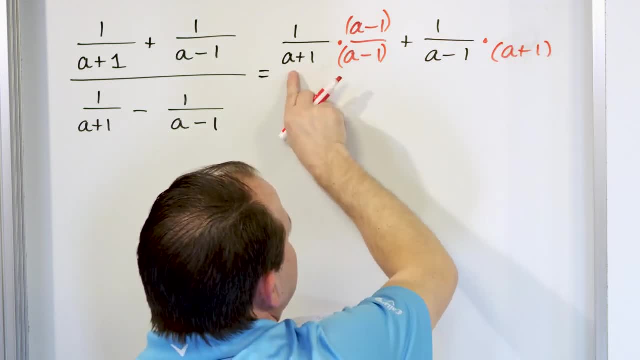 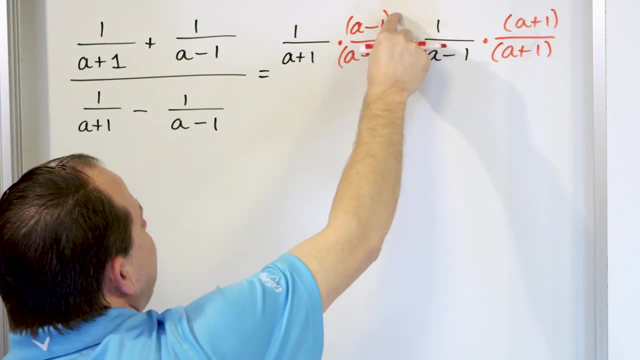 it match over here. I'm going to multiply by a plus 1, which is what this is- over a plus 1.. You see what's going on. All I've done is multiply this fraction by 1.. This whole thing is 1. This. 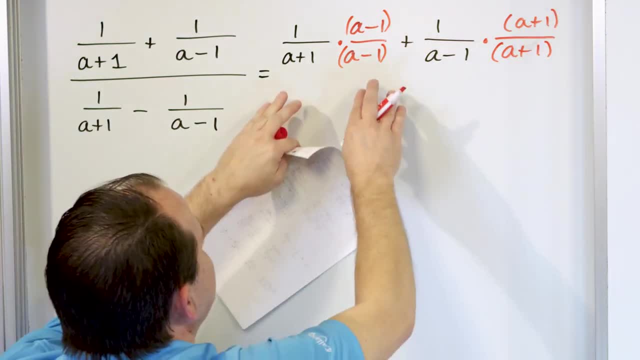 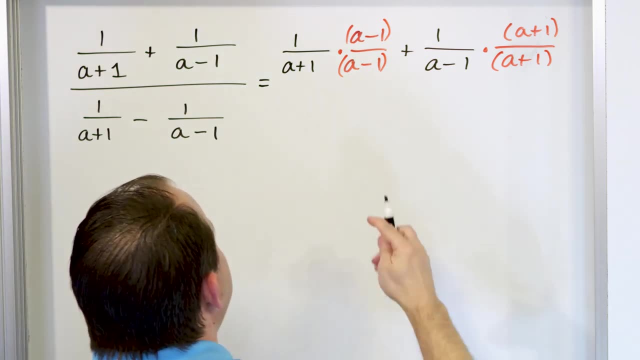 whole thing. divided is just 1 as well, so I haven't changed anything. but now the common denominators match. When I multiply this and I multiply this, they have the same bottom terms. So we'll leave that alone and we're going to come back to that in just a minute. On the bottom, we have to do the 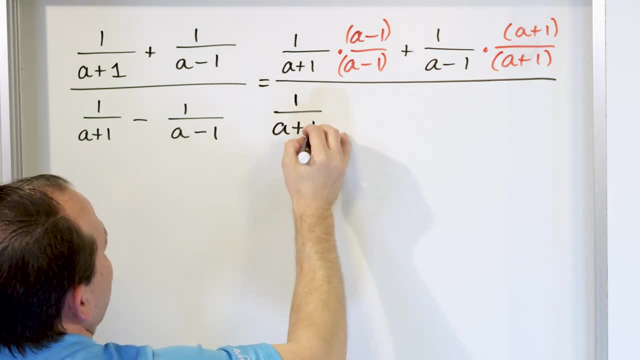 exact same thing down here. In fact, it's going to look exactly the same: a plus 1, and then I have now a minus sign, 1 over a minus 1.. So then I'll change colors, and it's literally going to. 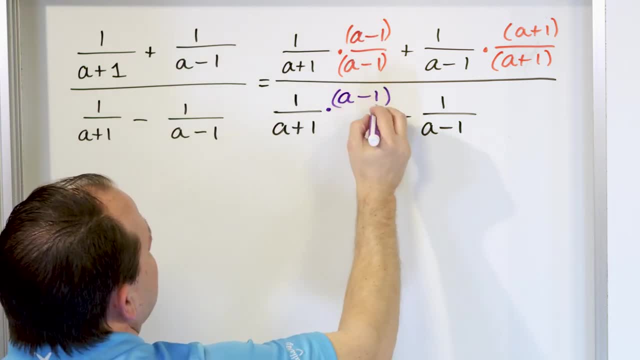 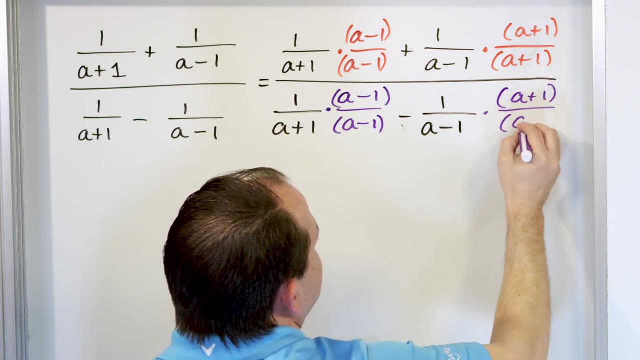 be the same thing. It's going to be a minus 1 over a minus 1, multiplied by a plus 1, a plus 1.. You might say, wow, that's a lot of work just to do this little thing. but that's just why. 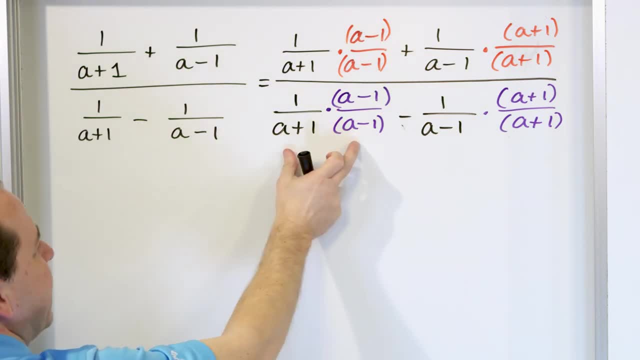 I'm telling you These are the hard problems, right? But now I have a common denominator here which will match this after I do the multiplication. So what we can do now is go ahead and tidy things up just a little bit to make sure you understand. So this whole thing multiplied together over here, 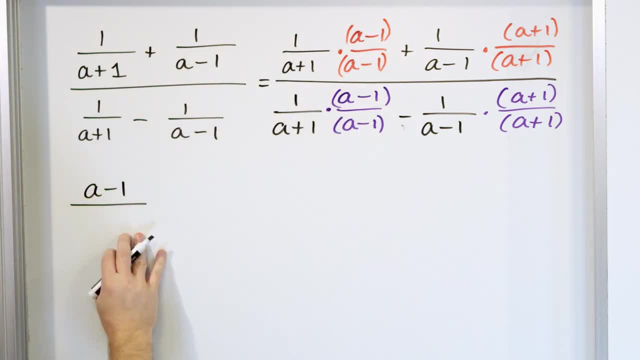 is going to give you in the top a minus 1,. right On the bottom you'll have the product of these two things. I'm going to wrap this in parentheses as well: a plus 1, a minus 1, and then I'm going to have to add to that over here 1 times. this will mean the numerator will. 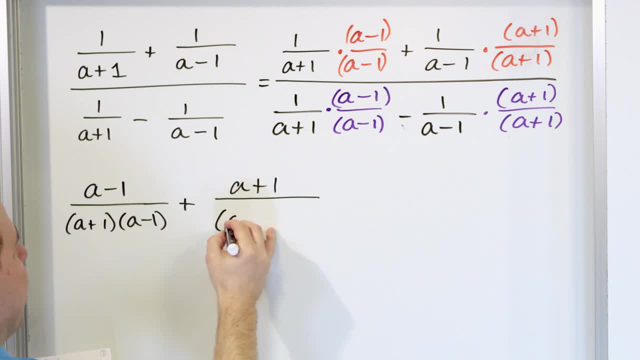 be a plus 1.. The denominator will be exactly the same. That was the whole point: a plus 1, a minus 1.. So now you see, I have a common denominator. I can add those, but unfortunately I still have this bottom thing. So it'll be the similar sort of thing. You'll have the a minus 1.. 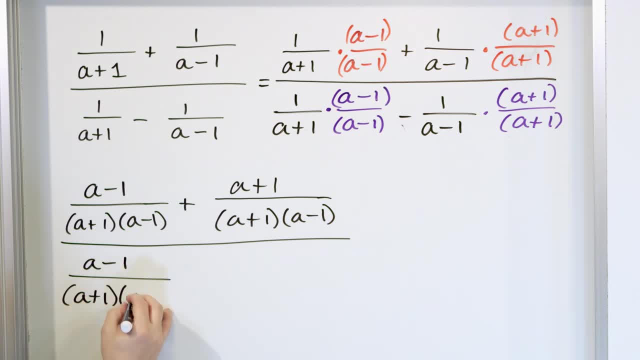 In fact, it's going to be exactly the same: a plus 1, a minus 1.. The only difference is this plus becomes a minus, a plus 1 over a plus 1, a minus 1.. Why did I rewrite it like that? Just so that you can clearly see. 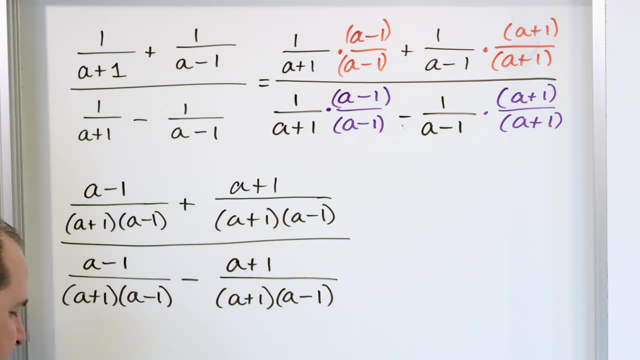 common denominator here. common denominator here. So then, in the next step, what can I do? It's going to be this term plus this term, right? So it'll be this term plus this term which will be- since it's a plus sign, it doesn't matter so much- with parentheses, like I was telling you. 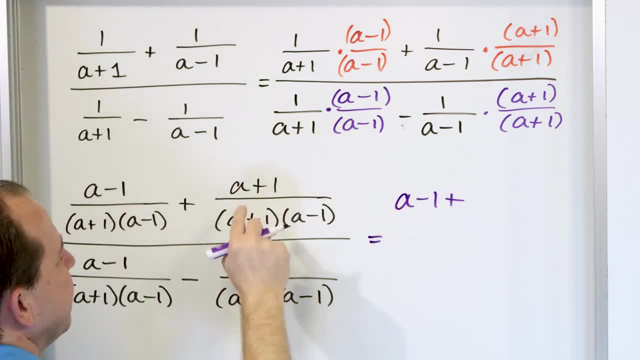 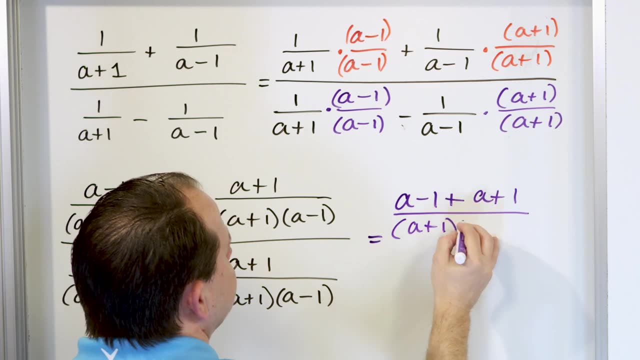 before. So just do it like this: a minus 1 plus this term, a plus 1.. The denominator here, this remains the same, which is a plus 1, a minus 1.. All you did was add those numerators together. 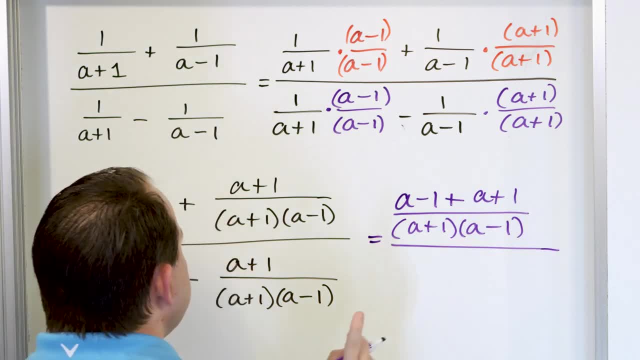 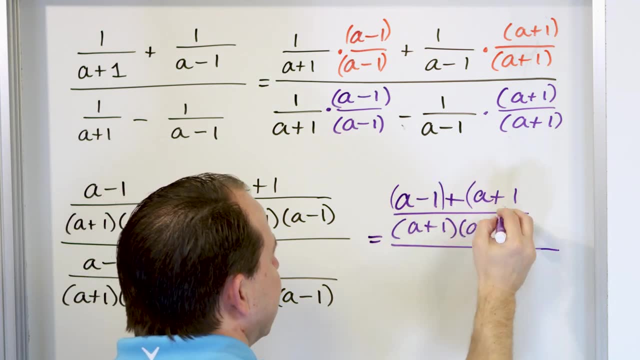 and you keep it over the exact same common denominator In the denominator. here you have to be a little more careful, In fact, because of this, I'm just going to make it 100% clear what you have here. Just go and wrap it in parentheses if you want to make it easy. The parentheses don't. 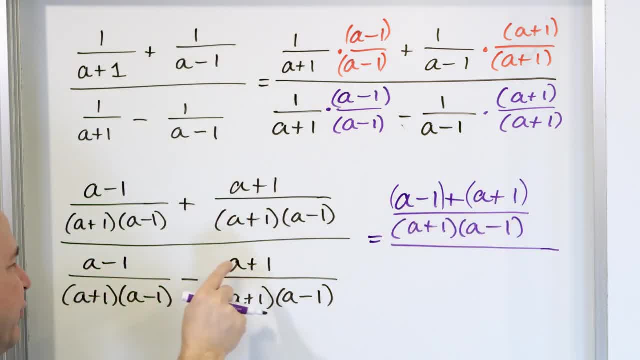 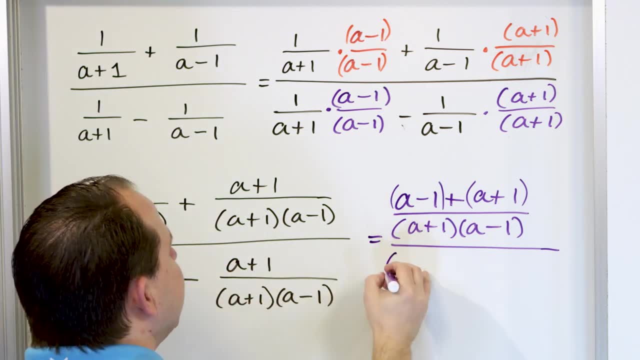 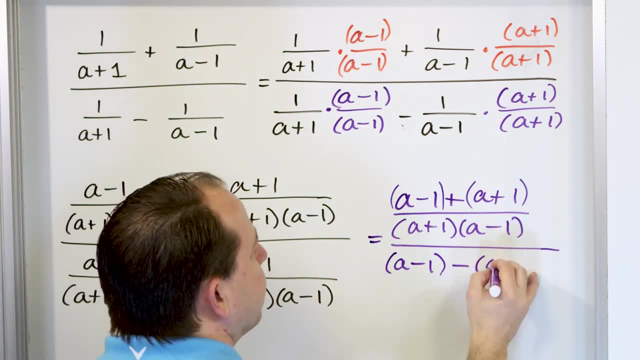 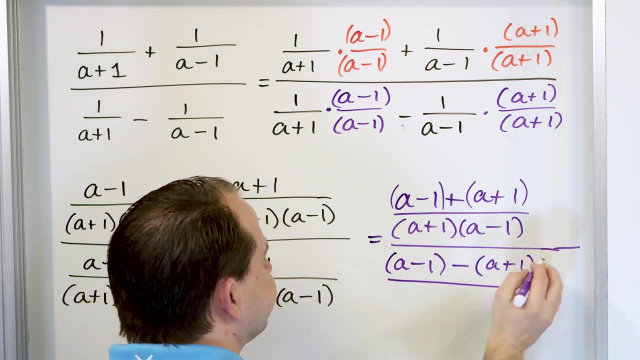 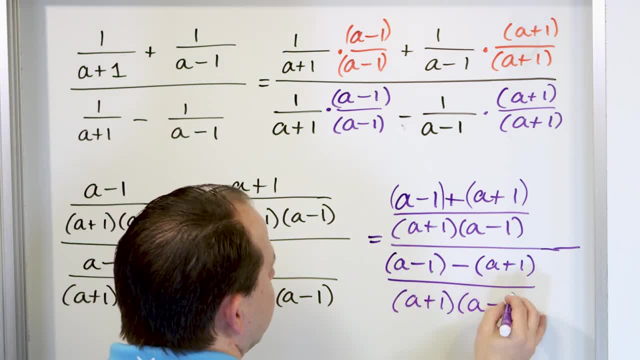 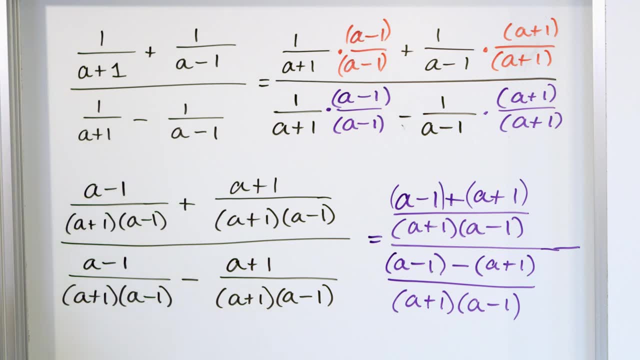 stays the same: a plus 1, a minus 1.. OK, So now I'm going to switch colors. We're going to go back to black, I think, And in the top what I'm going to have is a plus a. that's going. 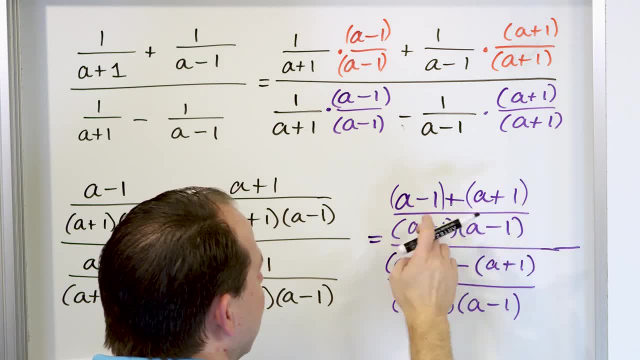 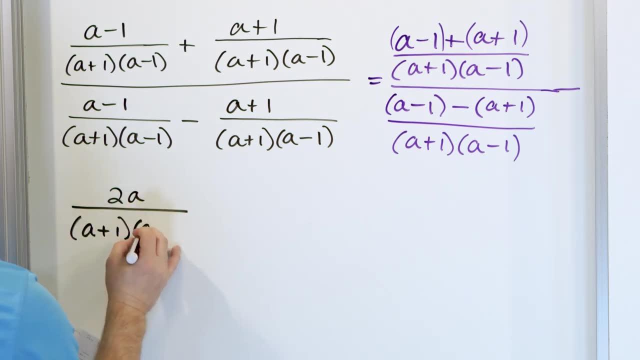 to give me 2a minus 1 plus 1.. That's going to give me 0. So all I have is 2a on the the top And the denominator here is a plus 1, a minus 1.. Then in the bottom: here I don't want. 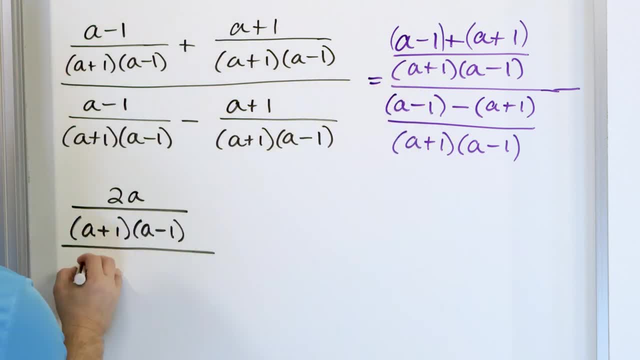 to make any mistakes. So I'm going to distribute this negative sign in: I have a minus 1, minus a minus 1, minus a minus 1.. Over here I will have a plus 1, a minus 1.. Now, what I'm going to do is: 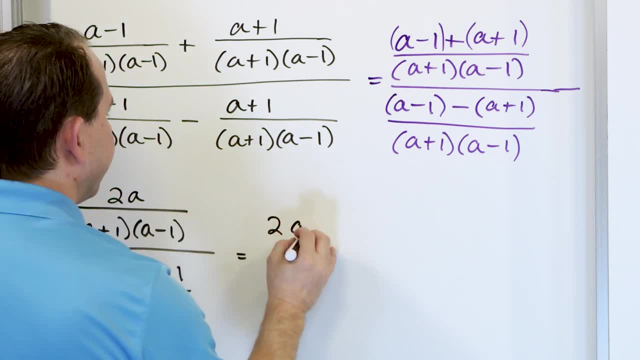 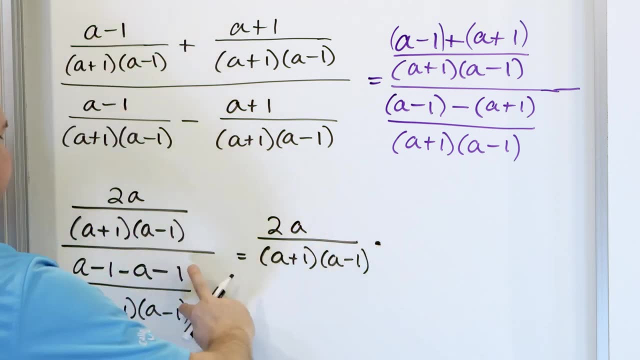 flip it over and multiply, So I'll have the 2a over, a plus 1, a minus 1.. Change this division to multiplication. Flip it over so this comes on the top. So it'll be a plus 1, a minus 1.. 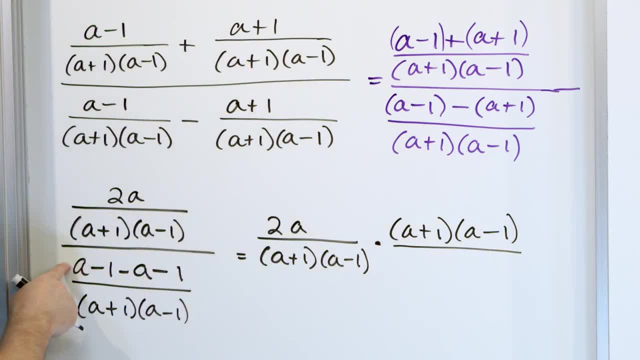 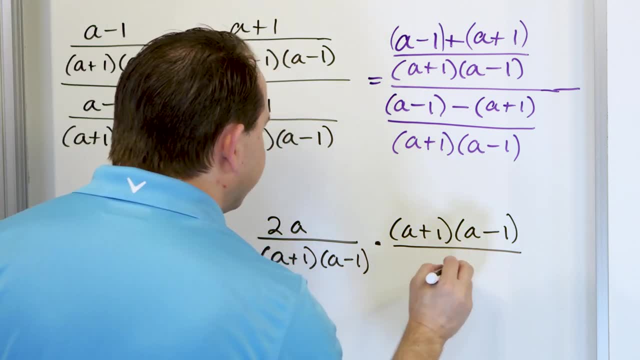 And the denominator is this. But here I can add this: a minus a is 0. So the a's go away. Negative 1 minus 1 gives you negative 2.. So here you're just going to have a negative 2.. Let me sync. 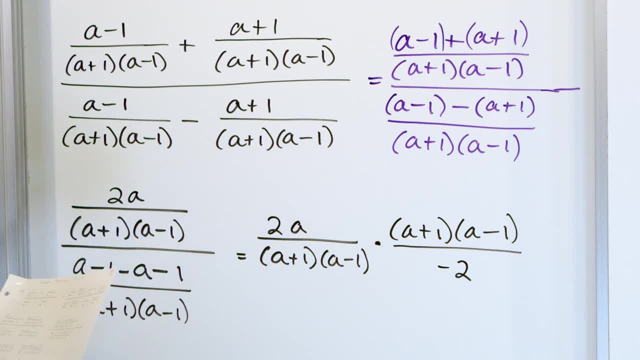 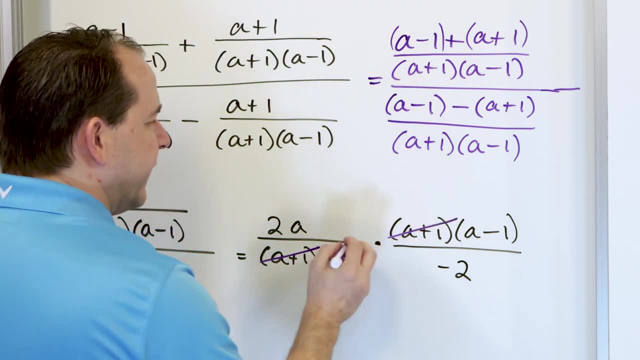 myself up and just make sure That I haven't made any big problems myself. So what I'm going to have, then, is nice cancellations. The a plus 1 completely cancels with this. Notice it's complete term. This cancels with this as a. 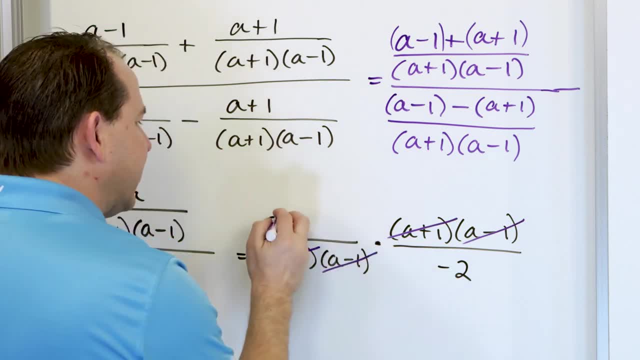 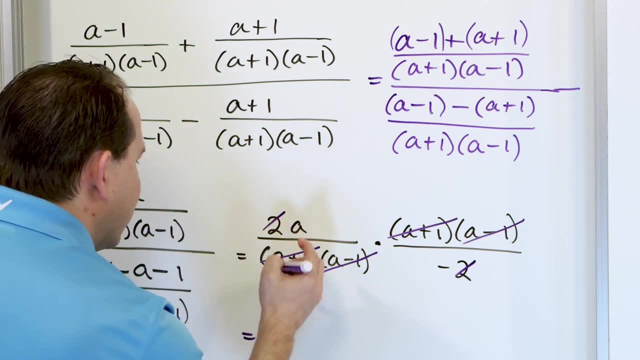 complete term And then the 2 and the 2 down here is going to cancel. I still have that minus sign, So I'm not striking through that. So really, all I have at the end of the day is going to be a on. 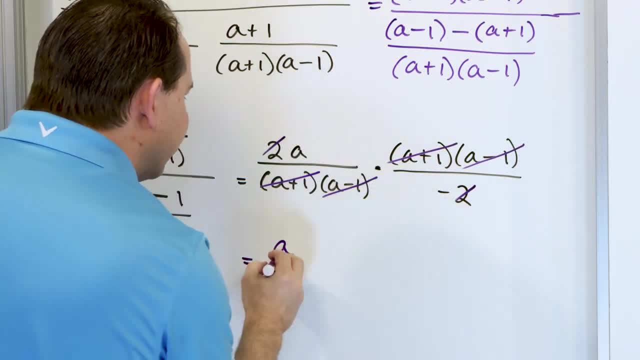 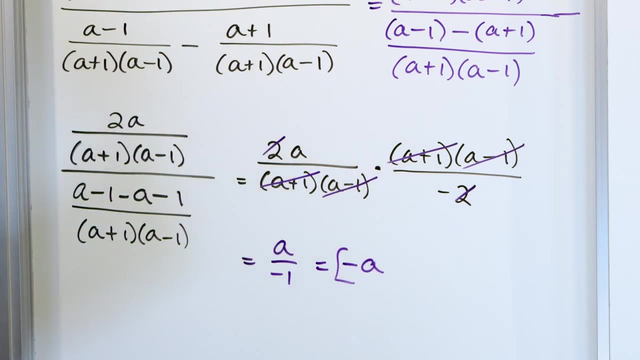 top a times 1, really, And then I have 1 times the negative 1.. So you have a negative 1. a times, or divided by negative 1. It's negative a. So all of that work just to get down to the answer, which is very simple. 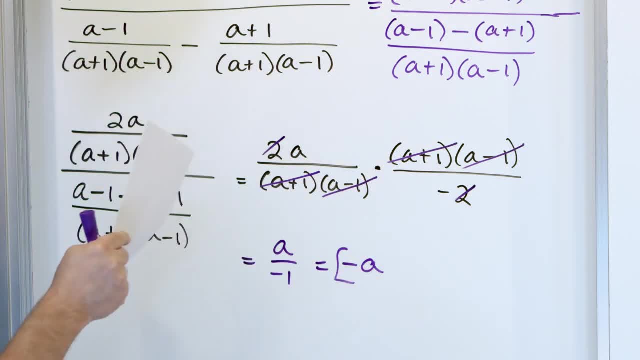 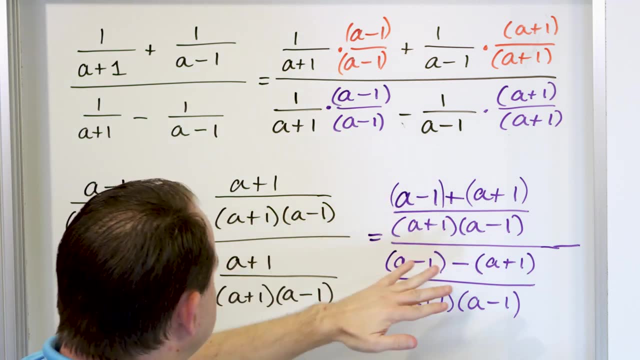 Negative a. But notice that, even though it was difficult, the same process applied: Find a common denominator, Find a common denominator, Get the numerators correct. Then do the subtraction, which we had to do. Keep the common denominators. Then we had to flip, multiply, cancel. I told you. 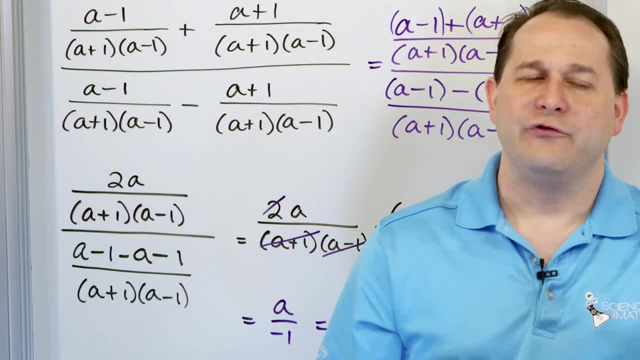 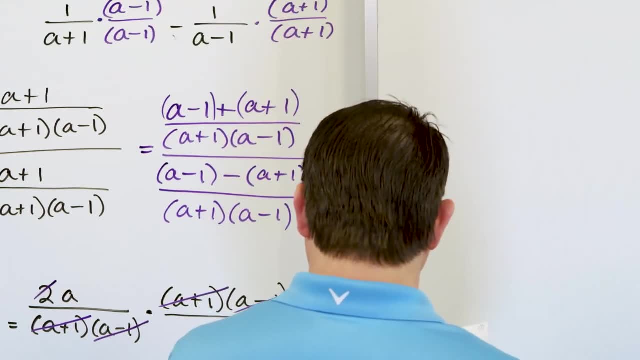 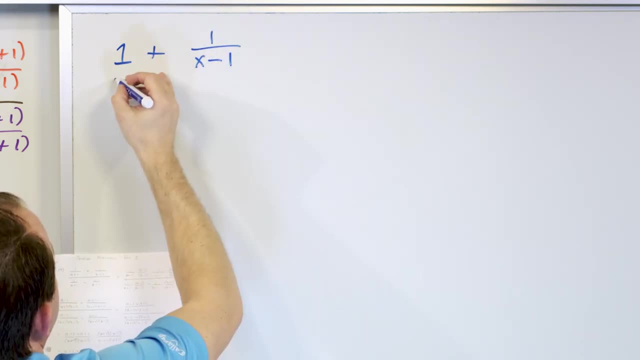 exactly that in the beginning of the lesson. It was all going to be the same song and dance, just with more tedium, so to speak. All right, Next problem: What if we have 1 plus 1 over x minus 1?? On the bottom we have 1 plus 1 over x squared minus 1.. 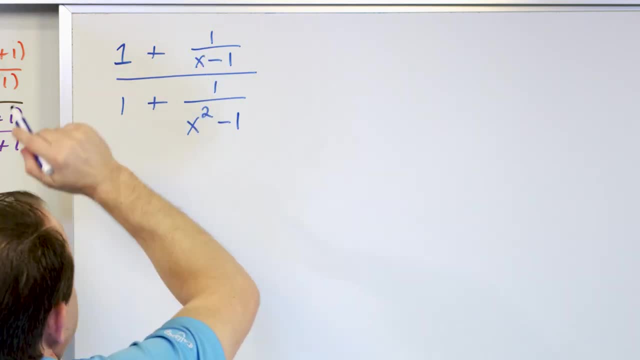 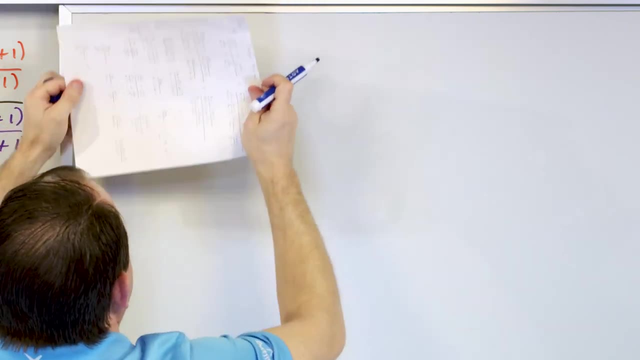 Looks very similar. So by now you should know you can't start canceling things. You have linked terms with pluses and minuses and all that. But you do see, I can try to add those fractions. I can try to add those fractions. So how do I do it? Well, this one's easier because I have ones here. 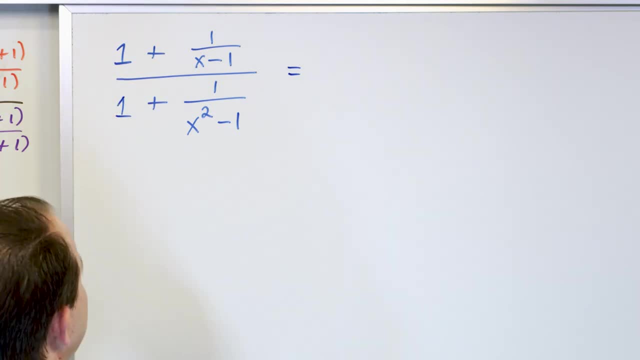 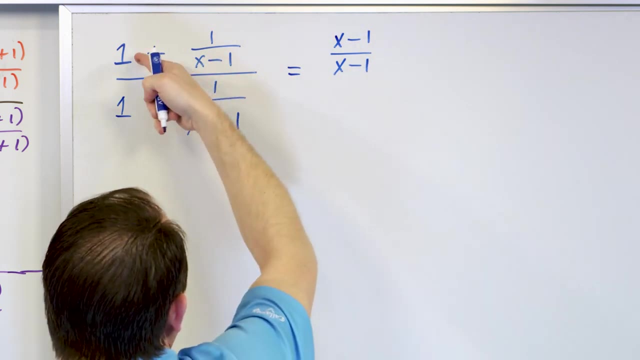 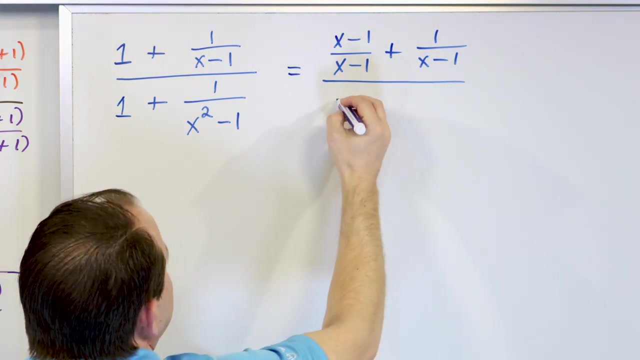 I can have lots of flexibility with the number 1.. Anything over itself is 1.. So since this denominator is x minus 1, I'll write this as x minus 1 over x minus 1, because that, after all, is 1, plus 1 over x minus 1.. In the bottom, I'll do the exact same thing, but this denominator is: 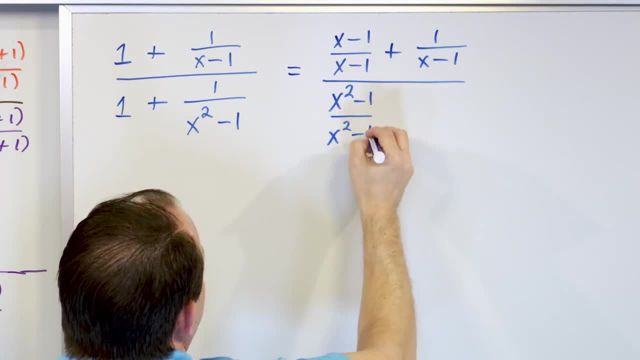 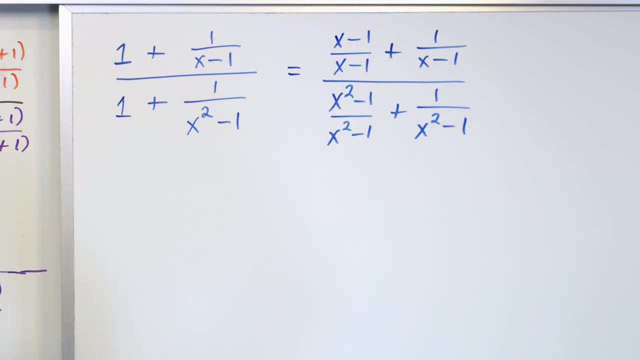 x squared minus 1 over x squared minus 1, because that, after all, is 1 plus 1 over x squared minus 1.. So it looks ugly, But it's actually not that bad, because now I have a common denominator. I'm going to add this, So: 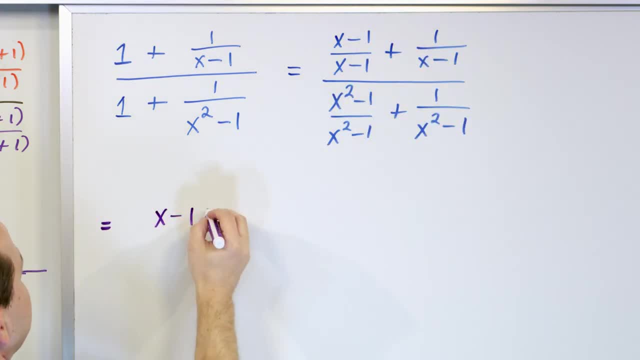 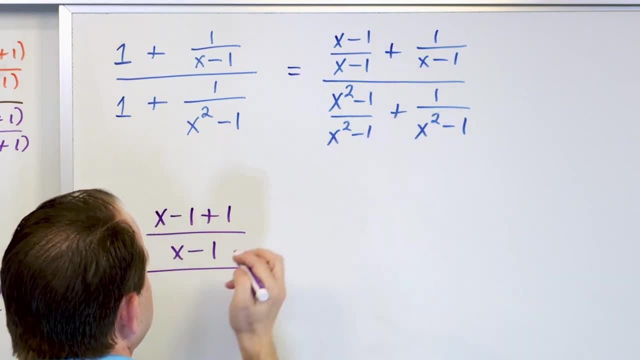 it's going to be this numerator plus 1.. So it'll be x minus 1 plus the 1.. The common denominator was x minus 1.. That's what's on the top. On the bottom, it'll be this plus 1, which is x squared minus 1. 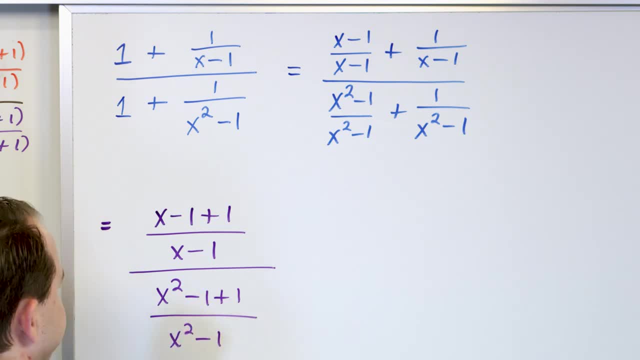 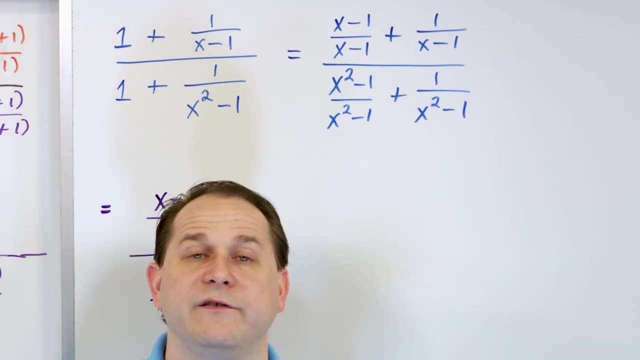 plus 1 over x, squared minus 1.. So you notice how I'm not doing the addition. I know that minus 1 plus 1 is 0 here in both cases, but I'm not doing it right now. I don't want to do too many things. 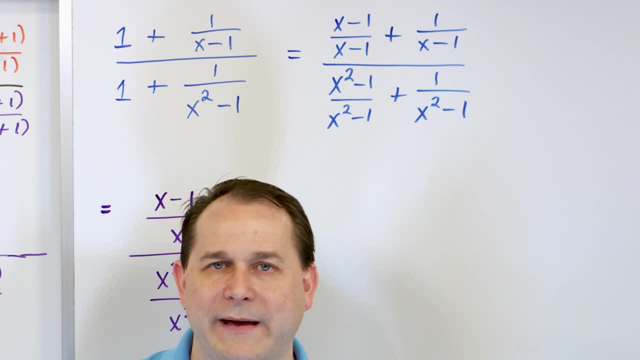 because I've done these a long time and I know that if I try to shortcut too many things I will mess it up. So I'm writing it down and in the next step I will say: negative 1, positive 1 is 0.. 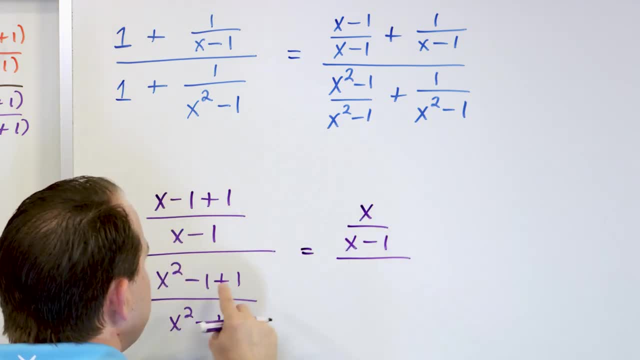 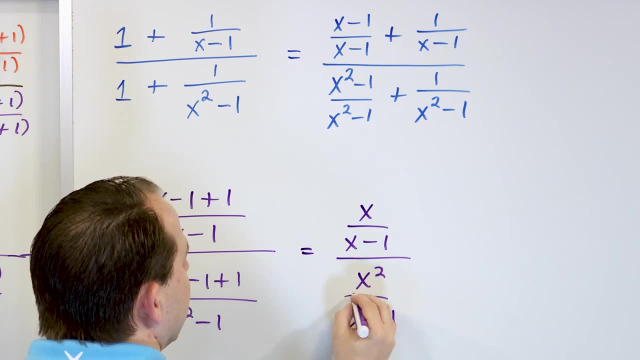 So it's just going to give me x on the top, x minus 1 on the bottom, Negative 1, positive, 1, 0.. So it's going to be x squared over, x squared minus 1, right, Then I can change this fraction. 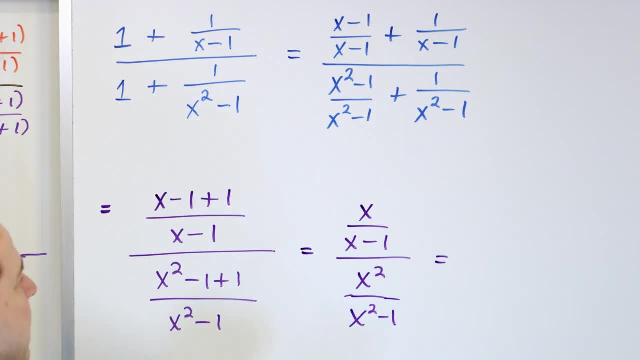 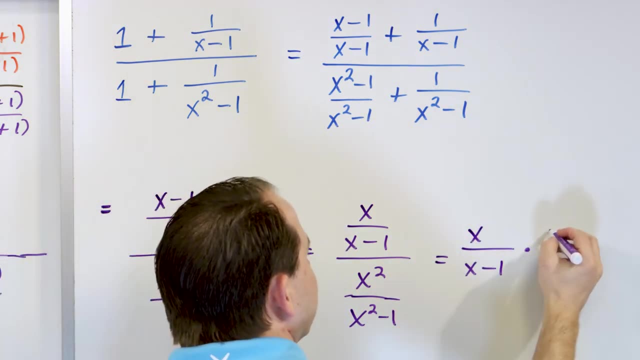 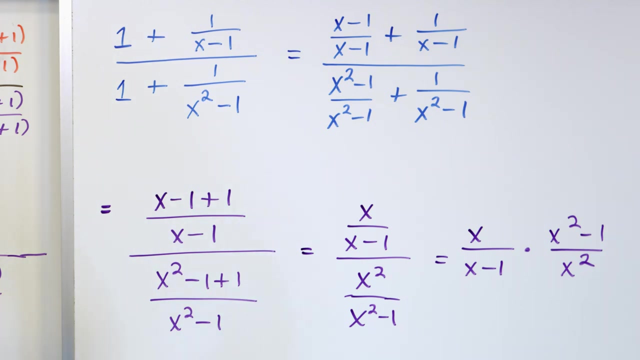 division to multiplication. So what will be is x over x minus 1.. Change this division To multiplication, flip the bottom fraction over x squared minus 1 over x squared, And immediately I start looking for things to cancel. I see, right away I have a single x which can cancel one. 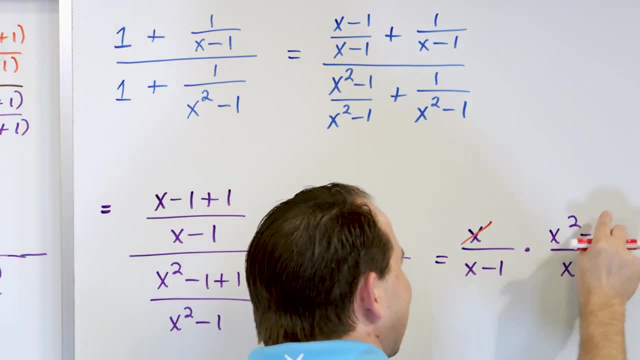 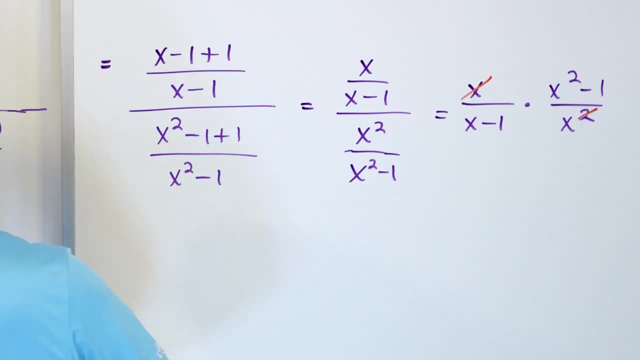 and only one of those. I leave one behind. You're tempted to try to cancel these, but you can't because they're not the same right. So we multiply the tops 1 times. this is going to give me: on the top, we're going to have x squared minus 1.. On the bottom, 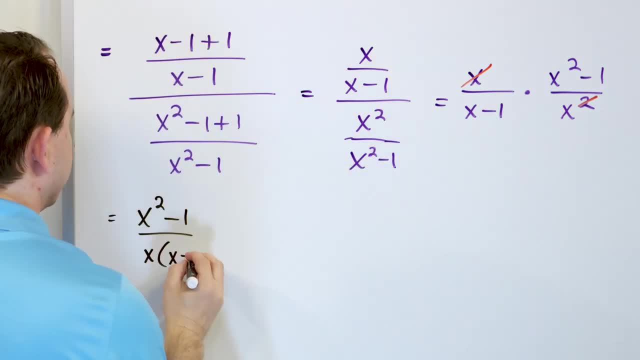 I have an x here, So it'll be x times x minus 1.. Now you're tempted to circle it, but then I'm trying to tell you over and over again: always look for anything that can be factored. This is difference of two. 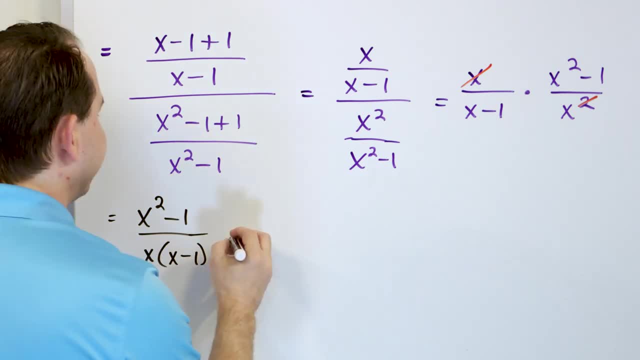 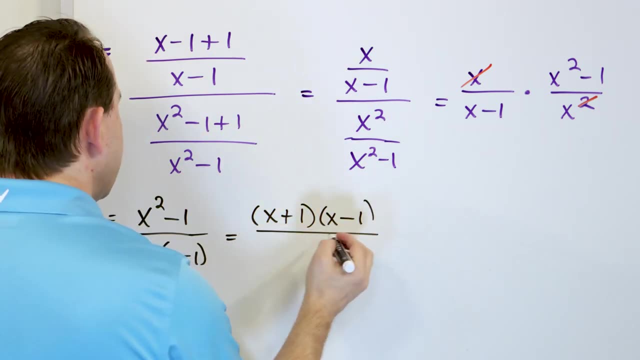 squares, x squared minus 1 can be x squared minus 1 squared, So I can write that as x plus 1, x minus 1.. Those multiply together to give me this: On the bottom I have x times x minus 1.. 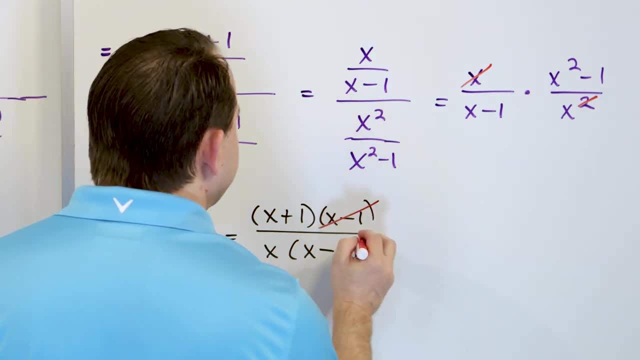 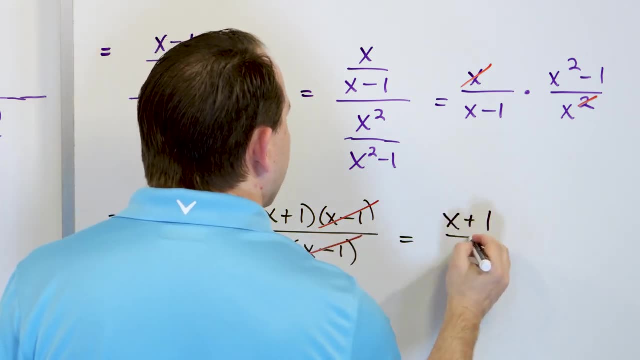 Now look at there. In the top and the bottom, I have something else that can now cancel. that was only revealed After the factoring was complete. So on the top, all I have left is x plus 1 over the bottom, which is just x, x plus 1 over x. There's nothing else to factor. There's nothing. 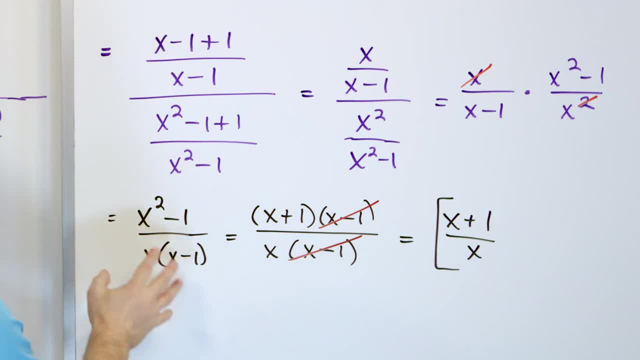 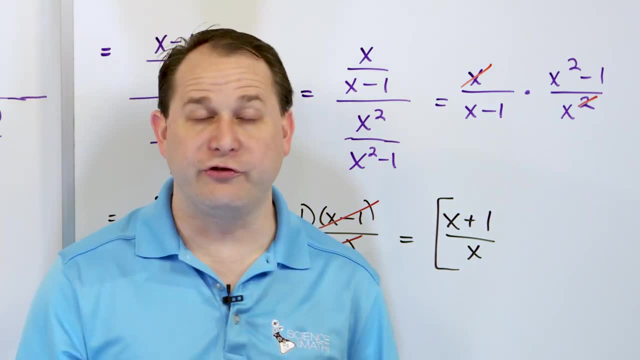 else. to simplify, That's as far as I can go. Anytime you have square terms anywhere, just try to factor it. In this case we could. So you see what I mean. This problem, if I gave it to you in the first batch, would be super, super hard and very confusing. We build 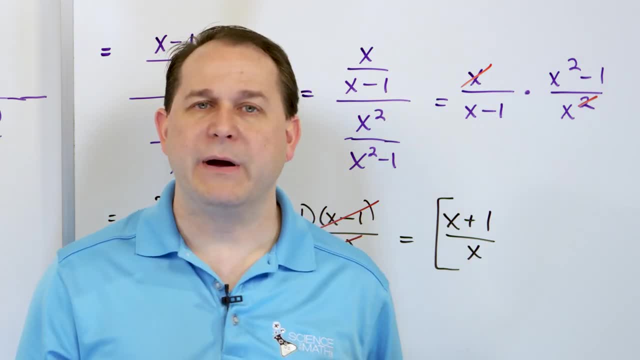 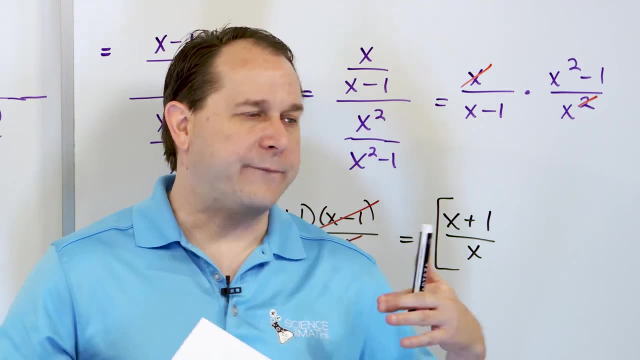 up our skills. Now it is difficult looking, but actually this process went pretty fast. It's because you already kind of know what to expect. We're going to find common denominators, We're going to add things, We're going to. 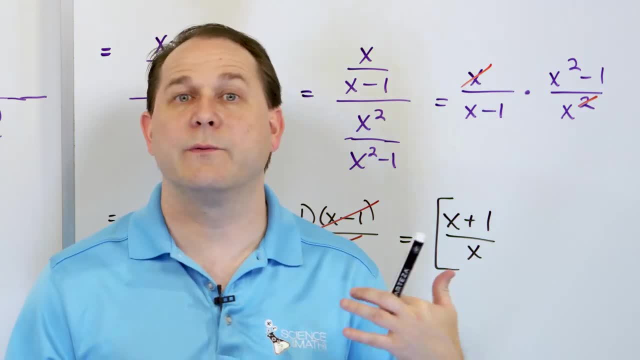 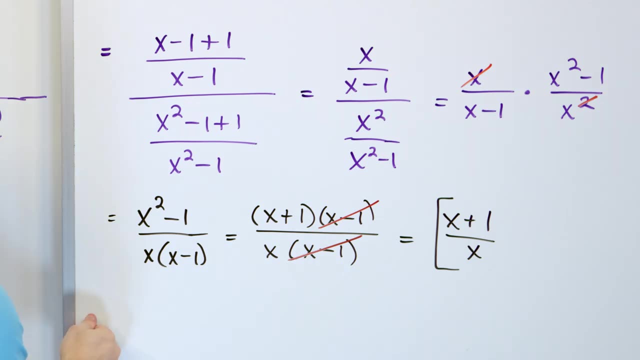 change the multiplication or the division to multiplication, Then we're going to cross, simplify, Then we're going to factor and simplify again, And I know I'm going a little faster, but we've done quite a few problems up to now, So I think I can do that. 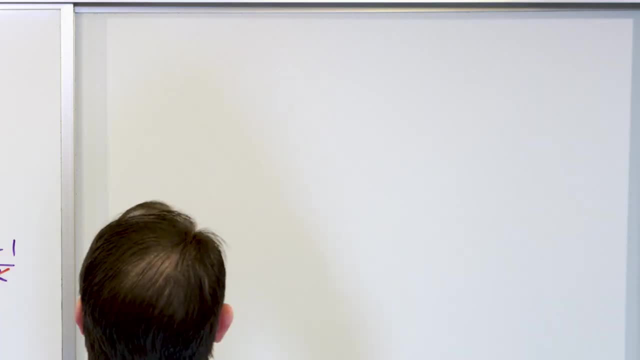 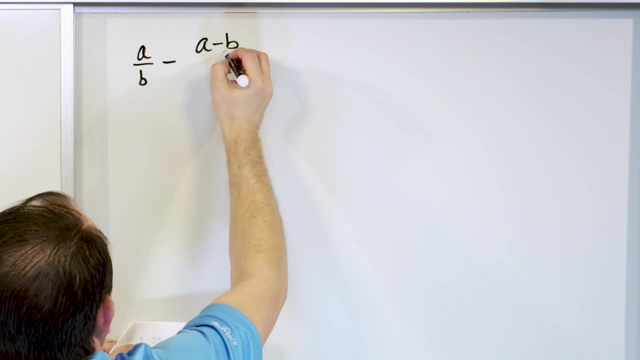 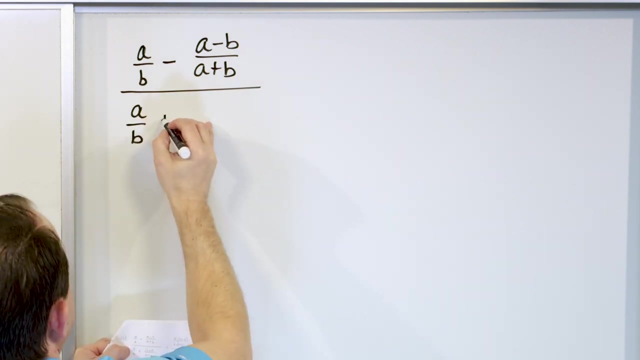 Only two more problems. This one looks like a monster at first, but we're going to get through it. What we have is a over b, minus a, minus b over a plus b. All of that is in the numerator. The bottom is a over b plus a plus b over a minus b Again. 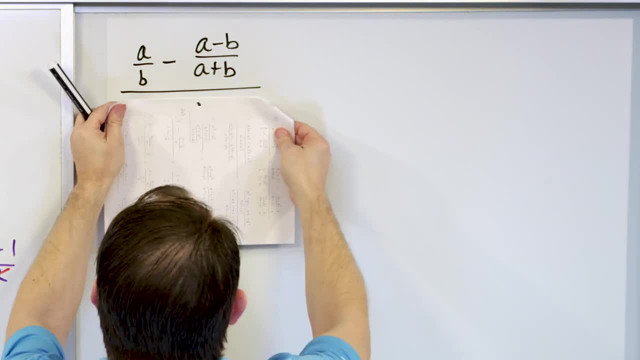 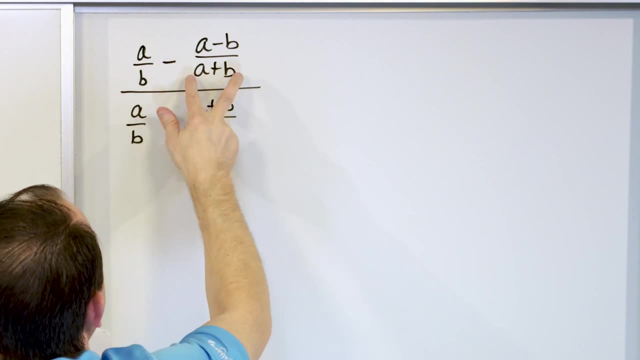 looks like a nightmare, right, But we just basically pretend the bottom isn't there. How do we get those fractions to be simplified? We have to have a common denominator. So I'm going to choose as my common denominator this times this, which means that what I'm going 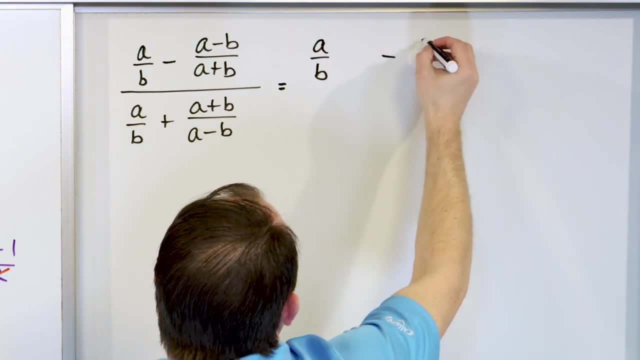 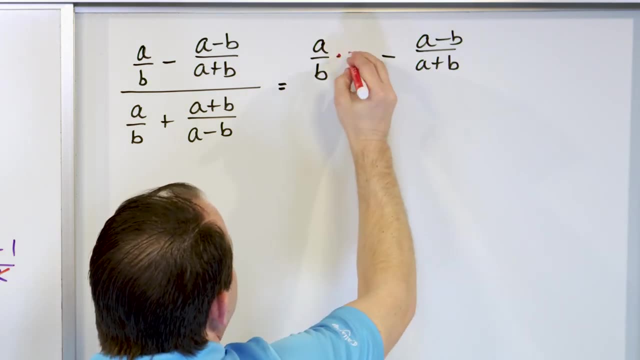 to have. I'm going to write a over b. I'm going to leave some room. I'm going to have a minus b over a plus b. So what I'm going to do is I'll multiply this fraction by the other denominator. 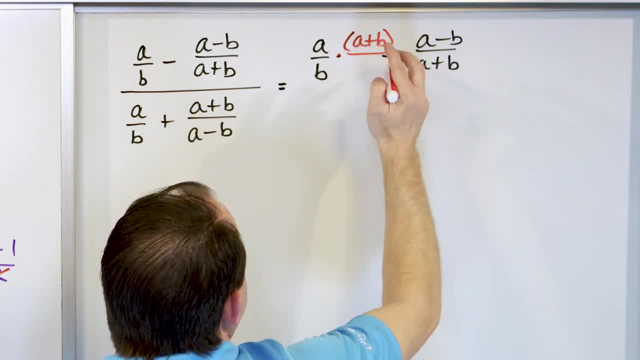 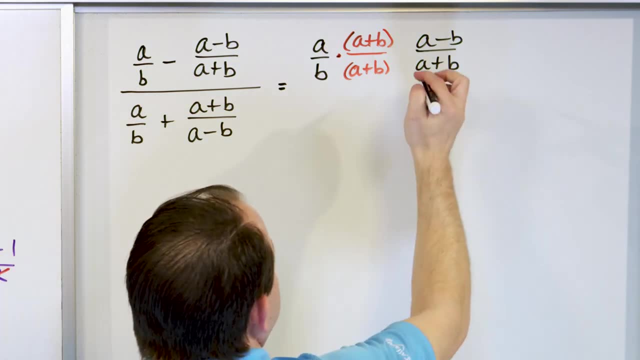 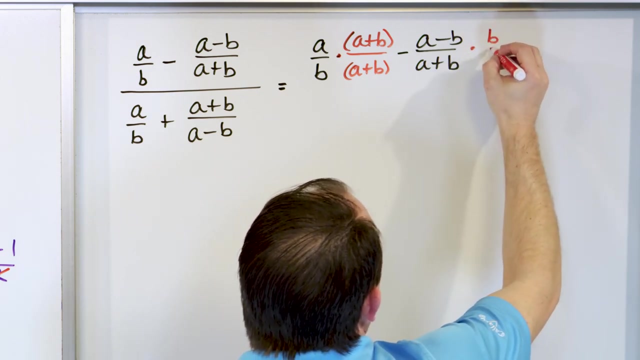 which is a plus b over. I wish I would have left a little more room. sorry, a plus b. Let me get rid of this minus sign here and kick it out just a little bit so we don't get in the way of each other. And then this one: I'm going to multiply this fraction times b over b Notice. 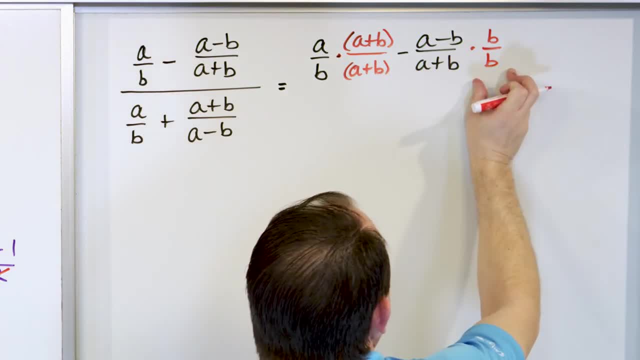 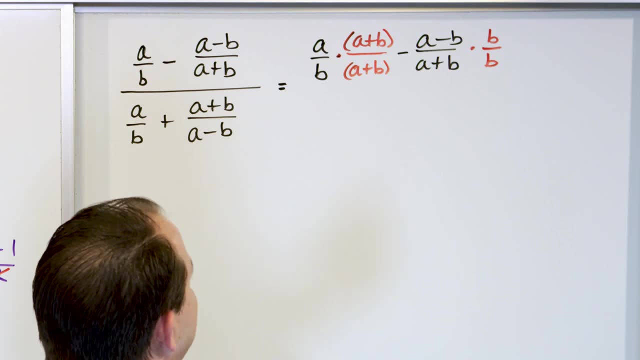 I'm multiplying this thing by one. I'm multiplying this thing by one, but this times this will give me b times a plus b. This times, this will give me b times a plus b. So I have the same common denominator. but I'm not going to start doing any of that yet. I'll save it for the next step. 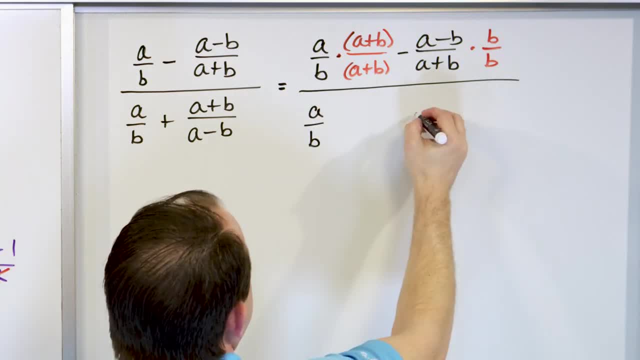 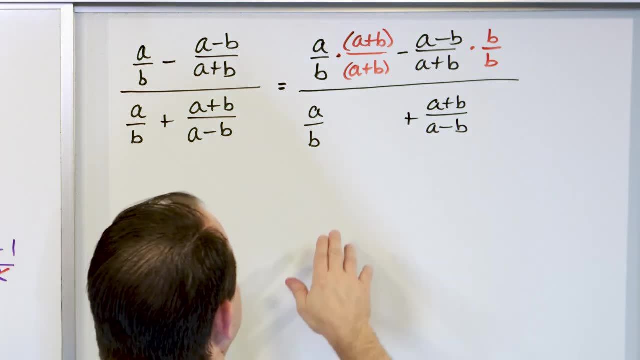 Down here I have the same kind of thing: a over b, leave me some room. plus a plus b over a minus b. Same exact thing. I'm going to choose as my common denominator to be the multiplication of those two, which means that: 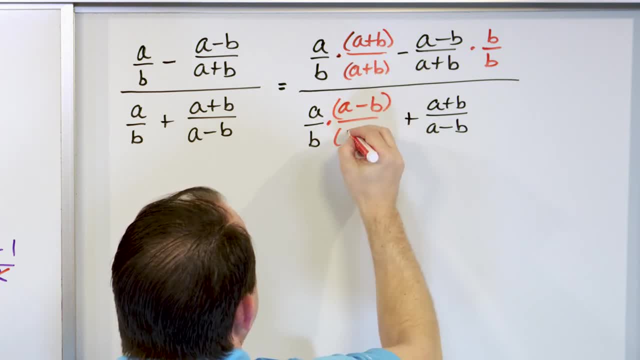 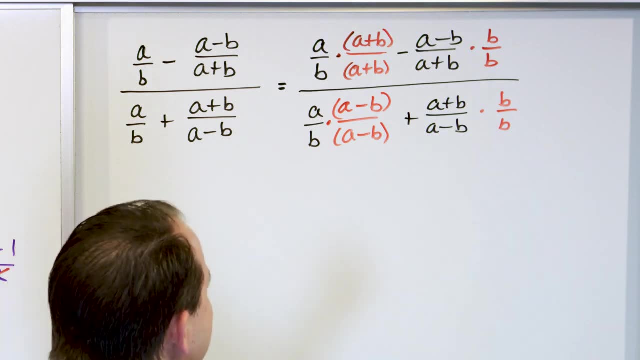 I'm going to need a minus b here, a minus b here, And then over here I will need b over b. Again. I'm multiplying by one in all cases, but now the common denominator is b times this and b times the. 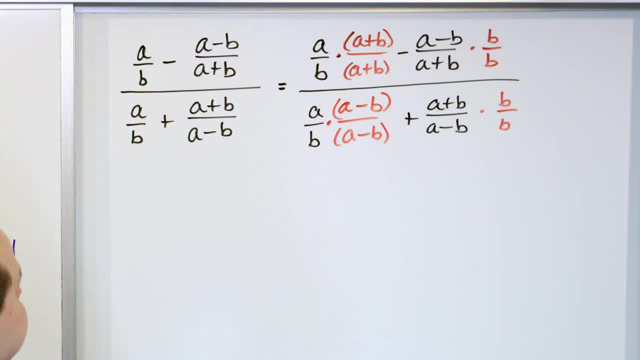 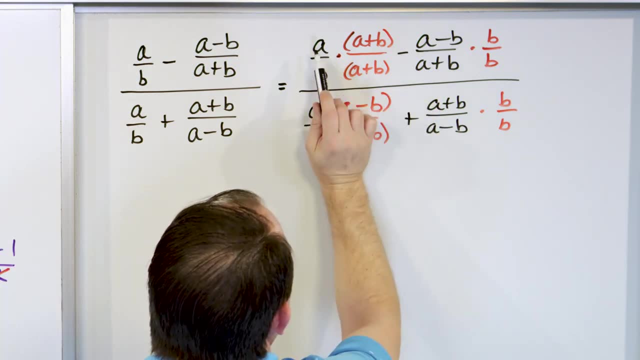 exact same thing. So I have common denominators everywhere, which is great. So here's where we have to be careful. right, We want to subtract these fractions. What you have in the numerator of this fraction is the multiplication of this minus this fraction, but this fraction is the. 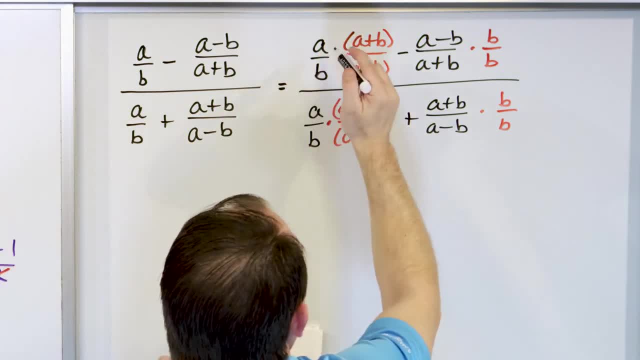 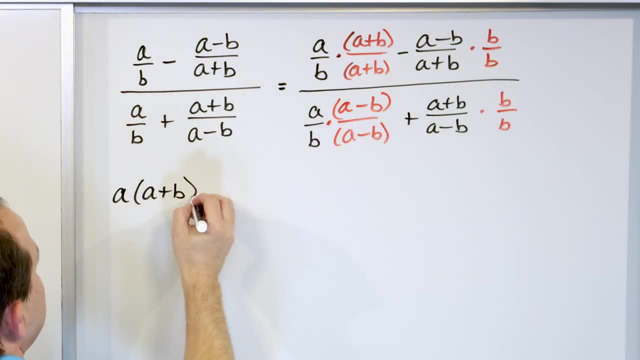 multiplication of this. So when we do all of the subtraction of the fraction, it's going to be this numerator minus this numerator. So you're going to have a times a plus b minus b, times a minus b, all divided by the common denominator, which is b times a plus b. Make sure you understand what happened there. It's this. 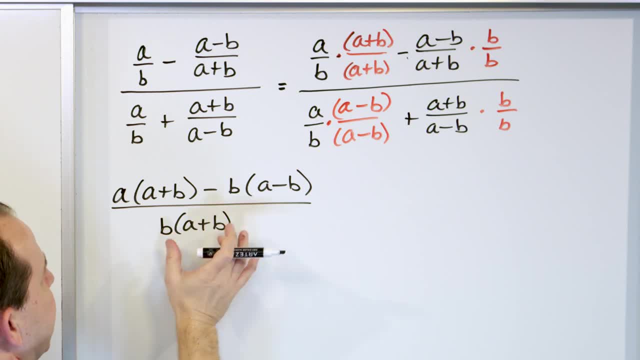 numerator minus this numerator. but you have to have things multiplied. The denominator is there. Then we will have a long fraction bar and it'll be exact same process here: A times a minus b plus this numerator, b times a plus b, over the common denominator, which is b a minus b. 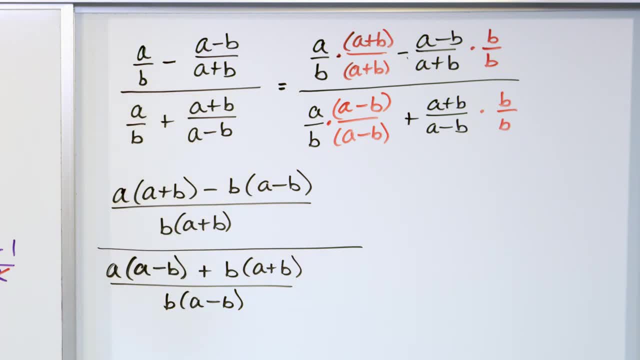 See what I mean. There's so many a's and b's and minuses, it's very easy to just kind of get lost in it here. All right, So then, what we have to do, you might say: well, I'm kind of confused, What do? 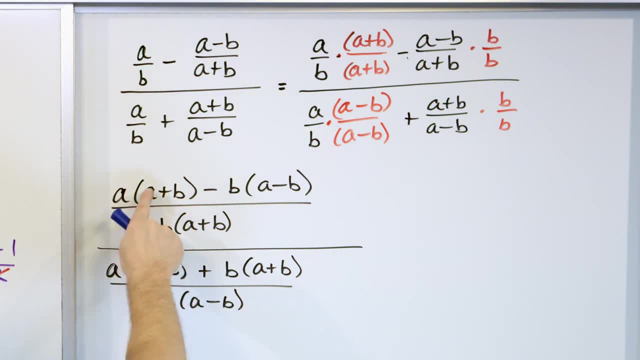 I do next. Well, you have a lot of things multiplied here and you have a subtraction and you have a lot of things multiplied. Here's what you're going to do: You're going to have a lot of things multiplied. We need to multiply all this out and then multiply all this out and then collect any. 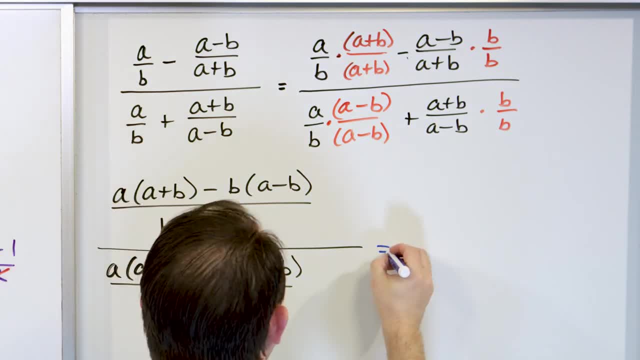 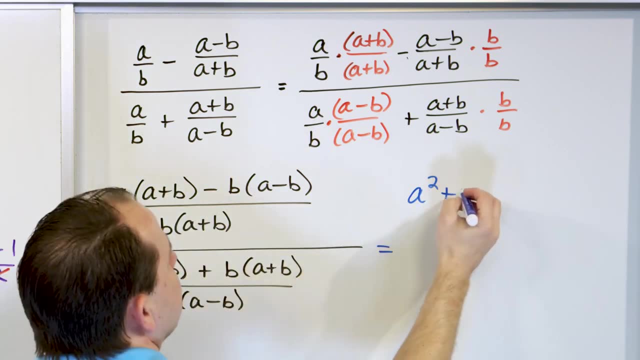 common terms there. So in the numerator it's just going to be a times. this is a squared. So let's do a squared plus a times b, right? Minus b times a. Let's write it as a times b, because I'm going to 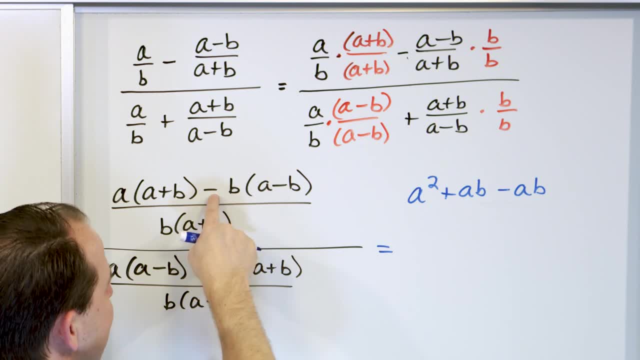 end up canceling it with this. So it's b times a. We'll write it as a b. Negative b times this, Then negative b times negative. b is positive b squared. You see what's going to happen. B's are going to. 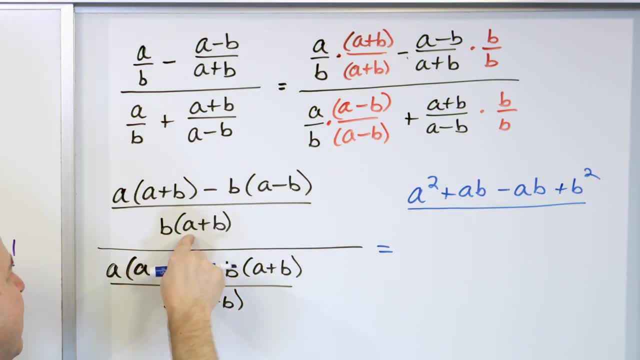 multiply. So you're going to simplify In the bottom. it is true that I could distribute this in, but I don't want to because I'm going to end up trying to cancel it later. In fact, if I'm not sure, I just leave it. 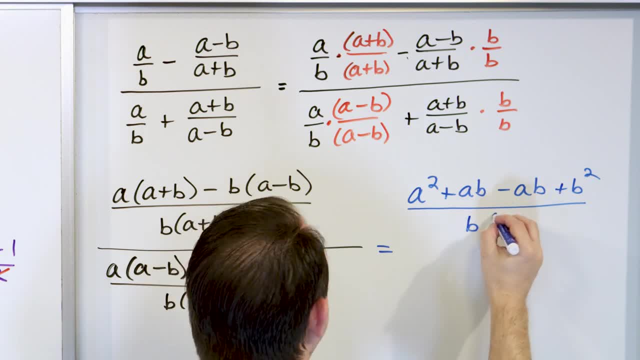 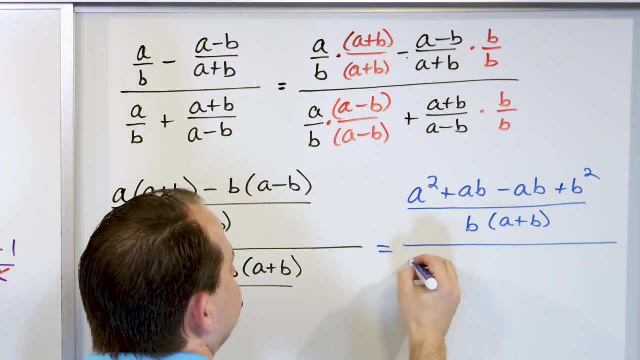 alone. I can do it later, right? So for now let's just leave it as b times a plus b. If I need to multiply that in later, I can do it In the bottom. I have a squared minus a b, A squared minus a- b. Then I have plus b a. 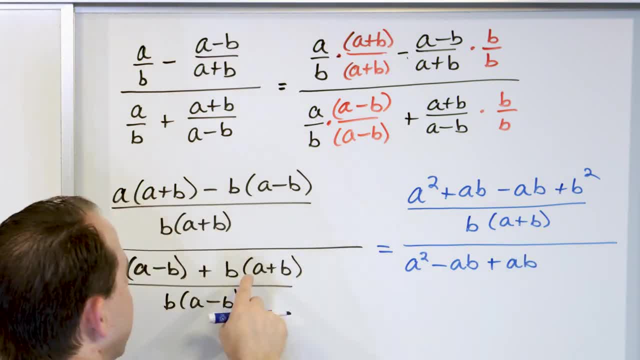 which you can write as a b B times b is b squared, So plus b squared. Notice again: I have a cancellation here. That's going to be nice In the denominator. I'm not going to multiply it in for now. I might do it later. b a, minus b. 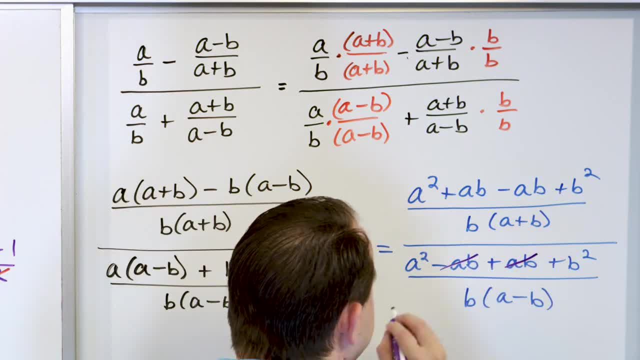 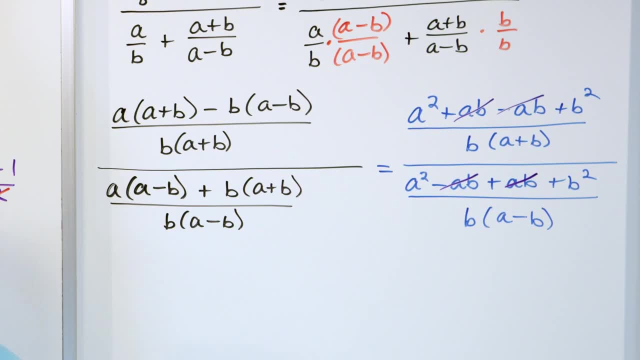 All right. So finally we get to some exciting part. The a- b can cancel with the negative a b giving me the zero. The a? b can cancel with the negative a b giving me zero there. So at the end of it- well, I shouldn't say it's the end of it. 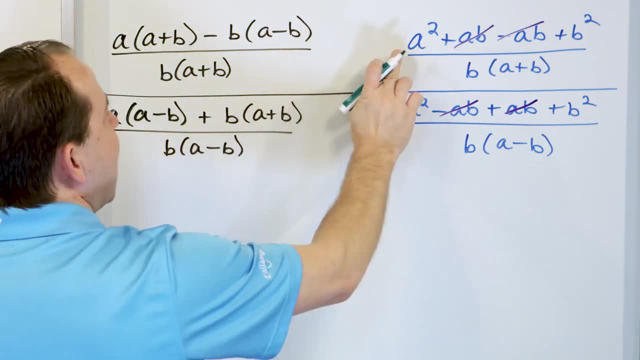 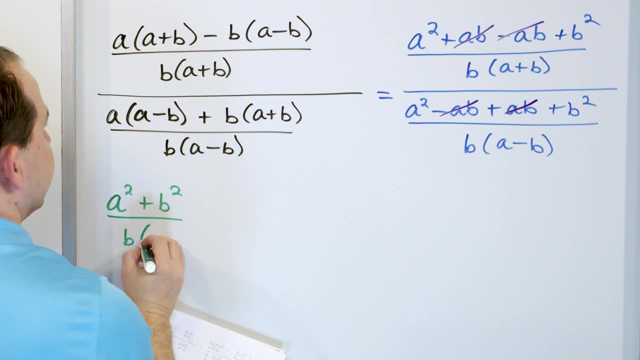 but basically this intermediate step here In the top you're going to have a squared plus b squared, a squared plus b squared over b times a plus b. That's the top fraction. The bottom fraction is a squared plus b squared. 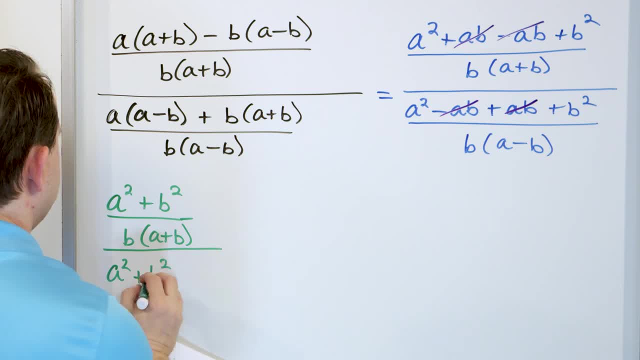 a squared plus b squared, The bottom fraction is, or the bottom denominator, b a minus b. Now you start to get excited because you see the a squared plus b squared is common. but we're going to take it step by step to make sure that we don't make any mistakes. This is going to change to fraction multiplication. 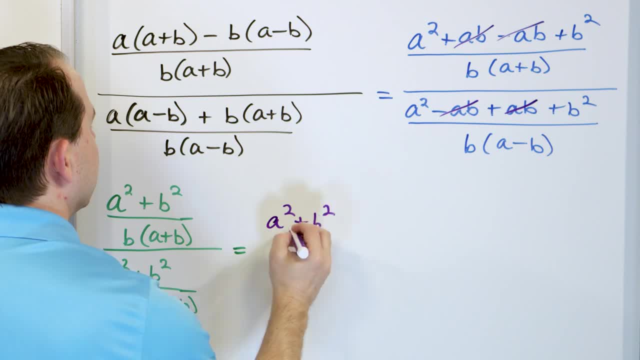 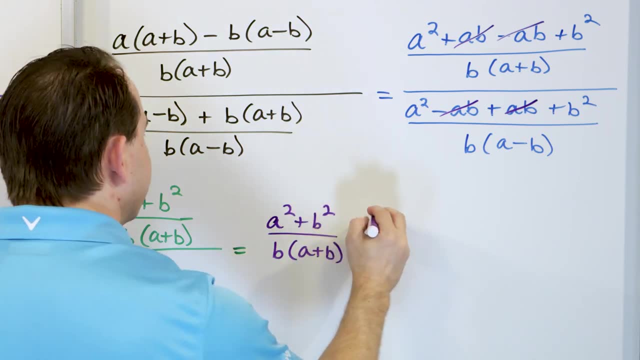 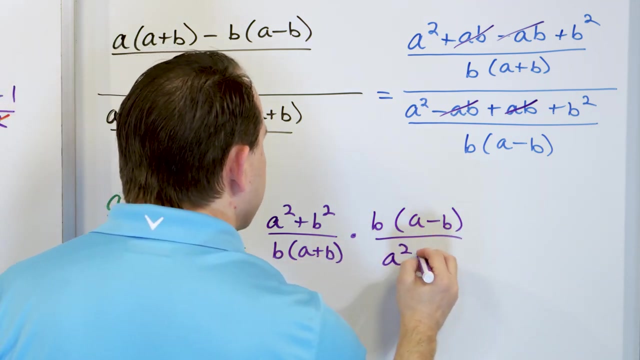 So what you have is a squared plus b squared over this: b a plus b. Change this to multiplication, Flip this over. You're going to have b a minus b On the bottom. you'll have this on the bottom, So you have a squared plus b squared. 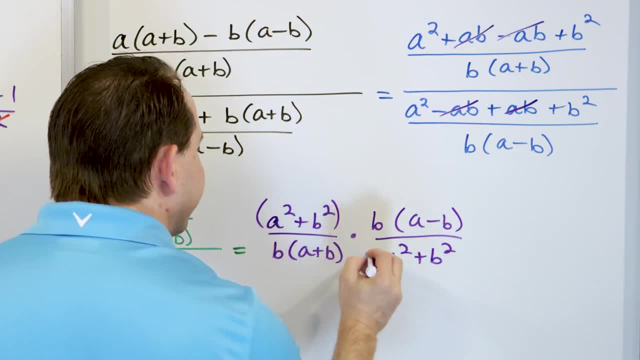 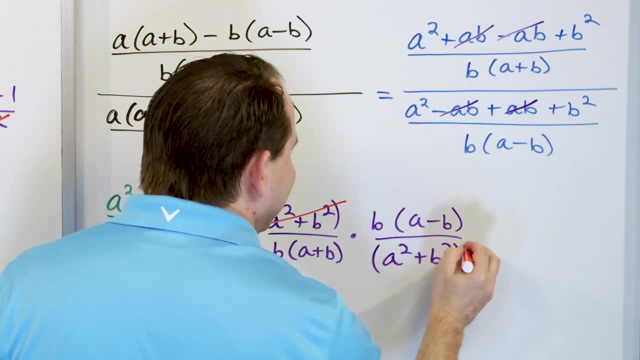 And again, you can always envision: numerators of fractions have an invisible set of parentheses around them, so to speak. If that helps you, Maybe it doesn't. So this entire term matches exactly this one And as a bonus, the b is out in front and it's factored out already, so I can cancel that with that. 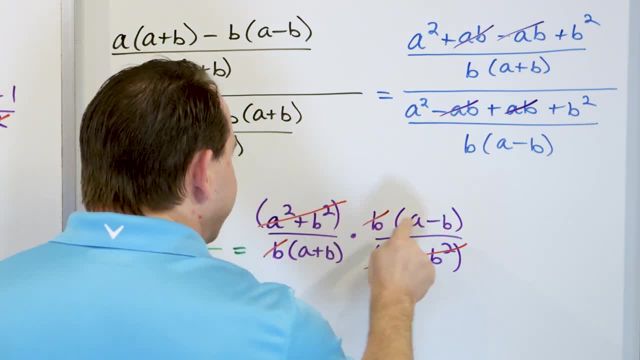 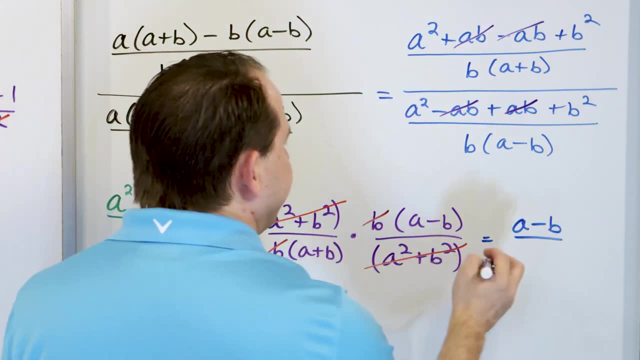 So all I have left is implied one times a minus b. So I have a minus b on the top And I have an implied one here times this a plus b. Now look at that: a minus b over a plus b. That's the final answer. 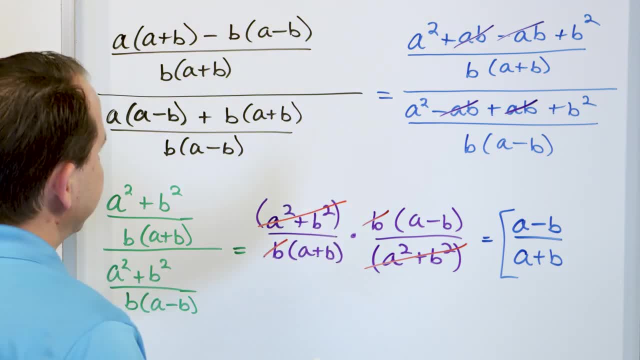 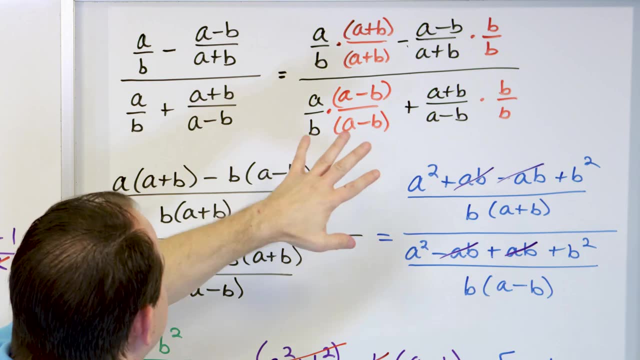 I know it looks crazy and it is crazy, but the process was the same. It's just more cumbersome because we had to get these common denominators And then, once we finally subtracted the fractions, we still had to distribute this stuff in. 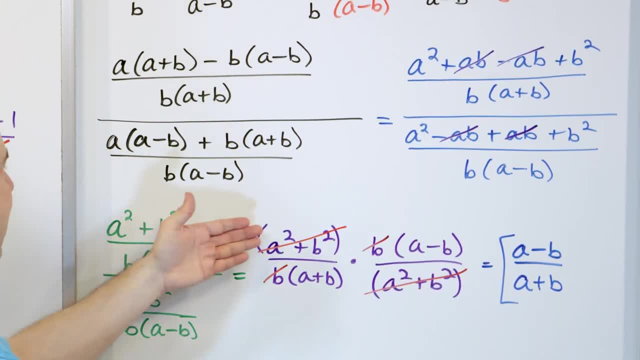 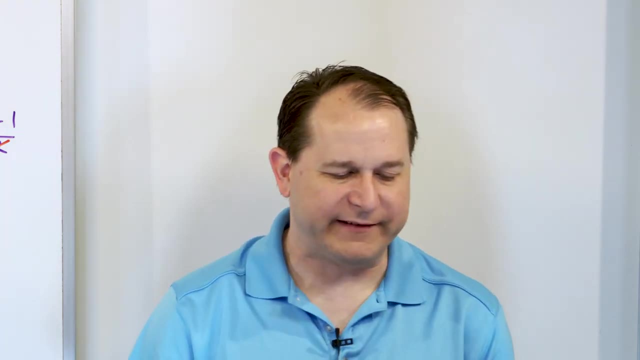 Cancel terms, simplify, and then we saw the giant cancellation that happened here at the end. But you cannot see these cancellations until you blow the terms out and then continue to simplify toward the final answer. Now, this last problem we're going to do. I almost didn't even do it because it's just such a crazy looking problem. 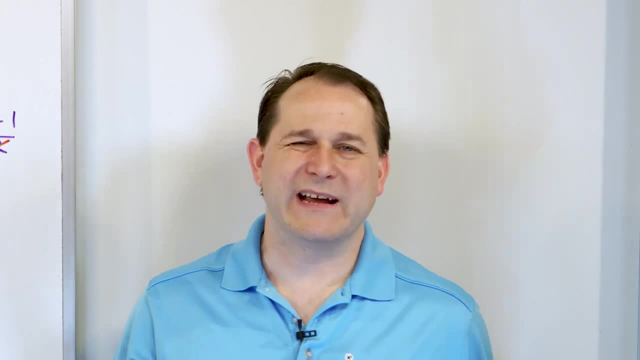 You know I'm like who would do? we really want to do every kind of problem, But really I find part of my job to sort of show you the easy problems, the medium problems, the hard problems and what we might call a challenge problem. 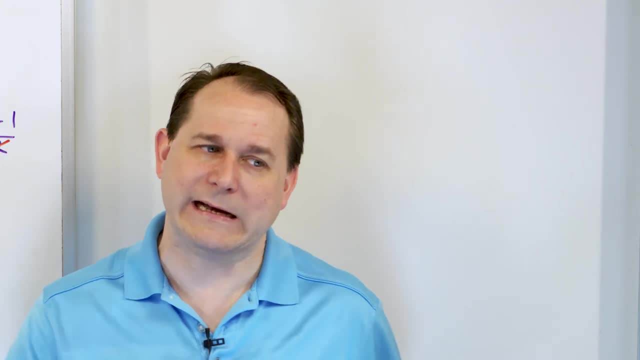 So why don't we do one challenge problem, just so I can show you how you would handle it And I don't think it's going to be too hard for you. We've conquered all of these little parts in all of the different kinds of problems we've done. 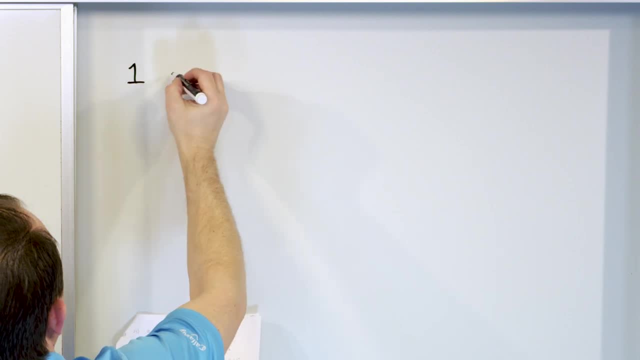 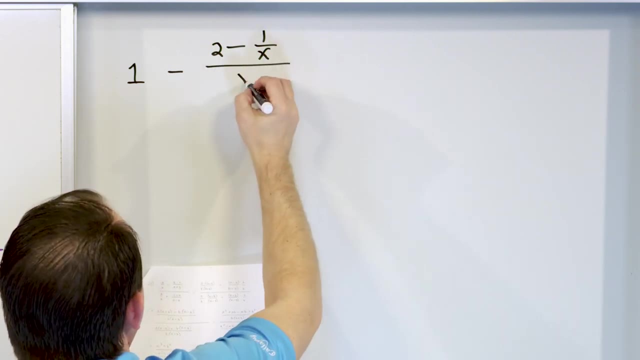 But this one still is a little challenging. Let's take a look. We have 1 minus. now check this out. We have 2 minus 1 over x, but we have this divided by x. So 1 is minus a fraction, but in the numerator is 2 minus a fraction. 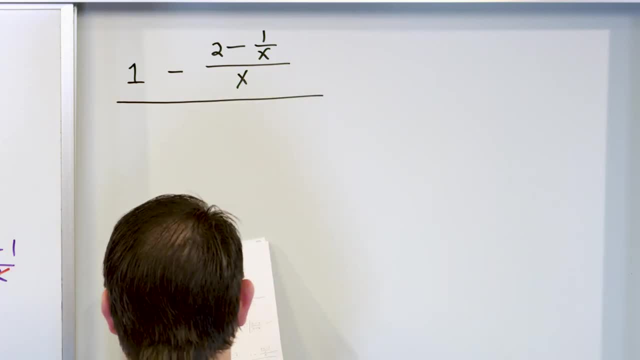 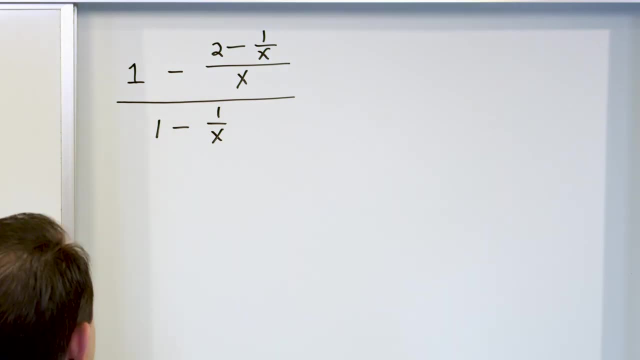 In the bottom. In the bottom is this: It's kind of crazy, But then that whole thing is divided by something else: 1 minus 1 over x. So you see we haven't done one quite like this. but how do you handle it? 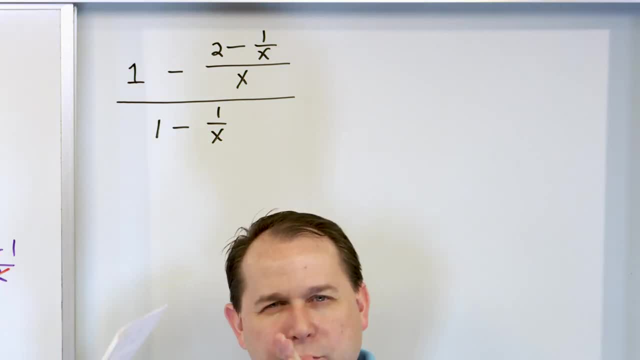 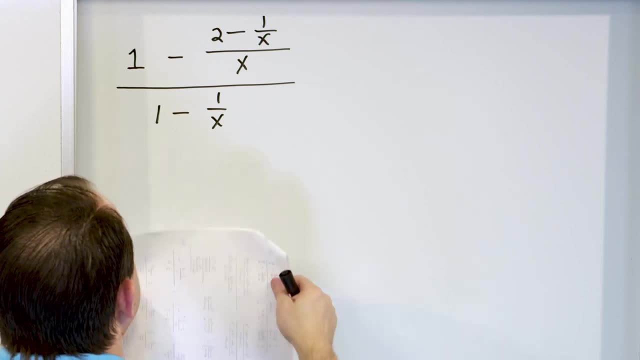 Right, It's just like you know the rules of order of operations: You go to the innermost parentheses. If you have multiple parentheses nested, you go to the most innermost and go out from there. So here, we're going to not only ignore the bottom, not only ignore this, but we're going to ignore that too. 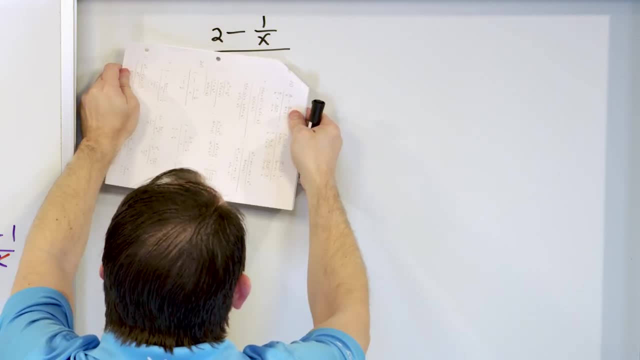 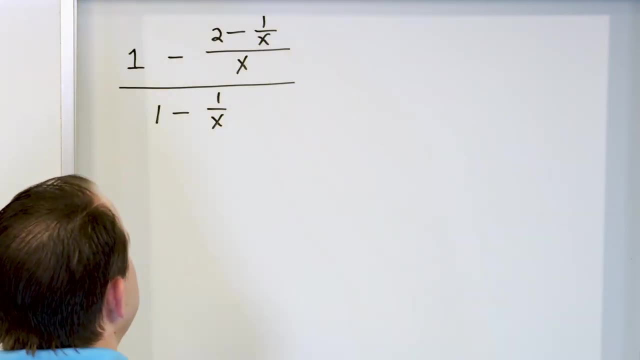 We're going to start by just simplifying that top thing. Once we get that done, we'll incorporate that bottom thing. Once we get that done, we'll fold in that 1 minus. Once we get that done, we'll do the bottom and we'll just kind of continue on like this. 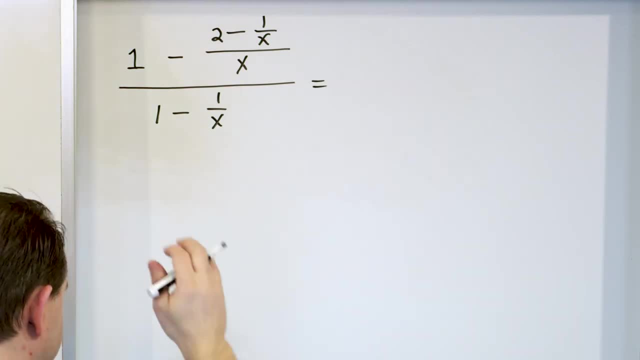 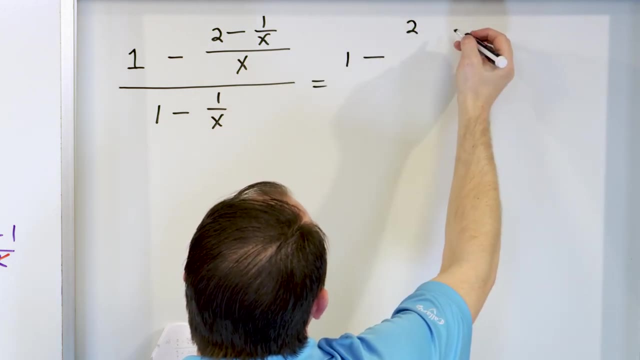 So it requires a lot of writing, but it's not difficult to do 1 minus In the top. what do we have? 2. Let's leave. Let's write it as 2 over 1, right? And then we'll subtract 1 over x. 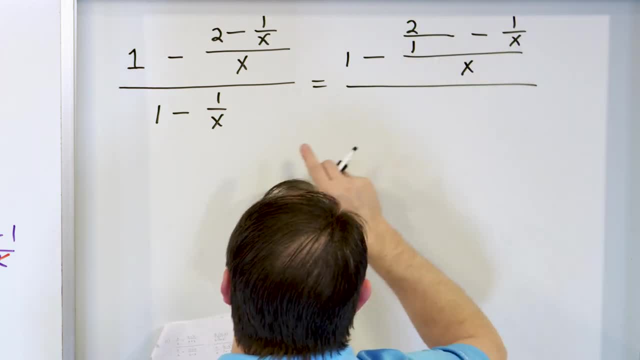 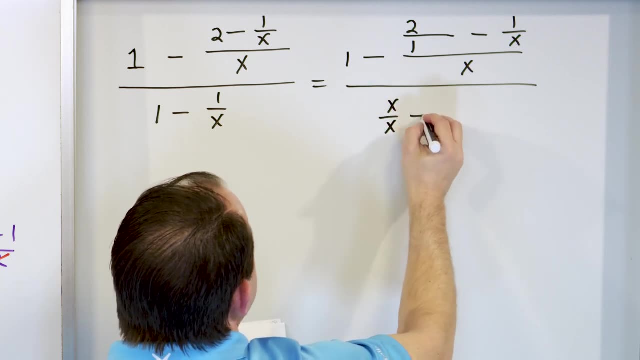 And then this whole thing is divided by x And then the bottom here We have. let's go ahead and work in parallel. really, Let's get a common denominator here. The 1 can be x over x minus 1 over x. 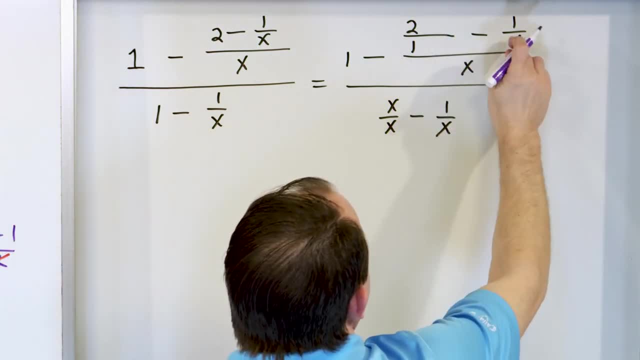 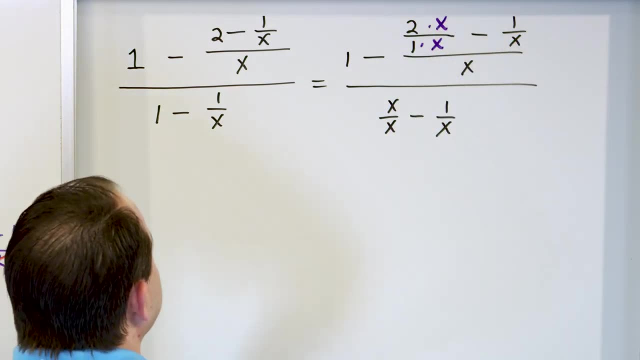 Now we didn't do the common denominator just yet. in the top We want 1 to be able to subtract this fraction. So we're just going to multiply by x by x, because then I'll have a common denominator here. So what do I have? 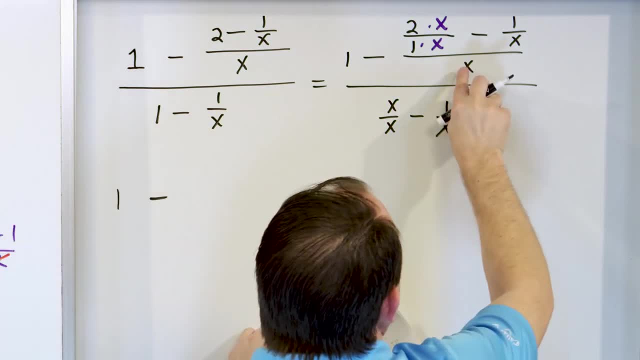 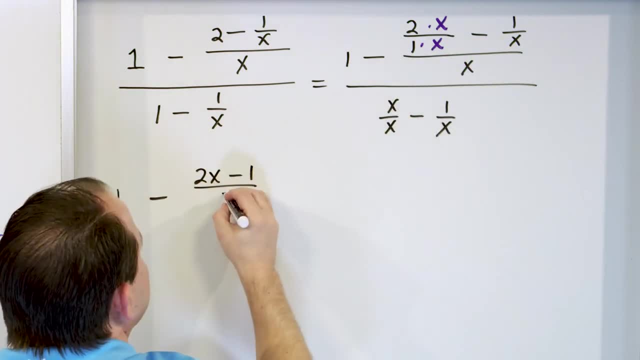 So it would be 2x minus 1.. So it would be 2x minus 1.. So it would be 2x minus 1.. For the numerator, the denominator is just x. It comes along for the ride And that whole thing is divided by x. 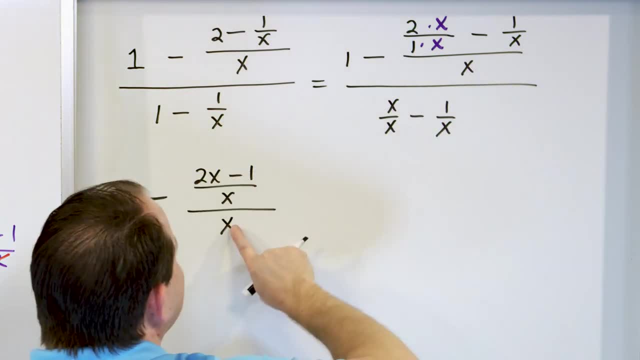 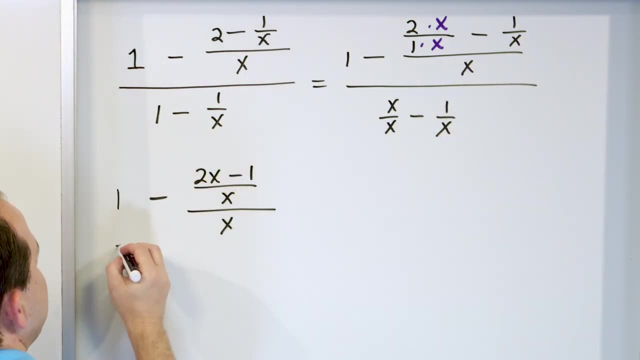 Notice we've done the fraction subtraction but this denominator of x stays there. This one comes from this denominator, So it's over x and then over x, kind of. again On the bottom here, x minus 1 over x common denominator. that we got all right. 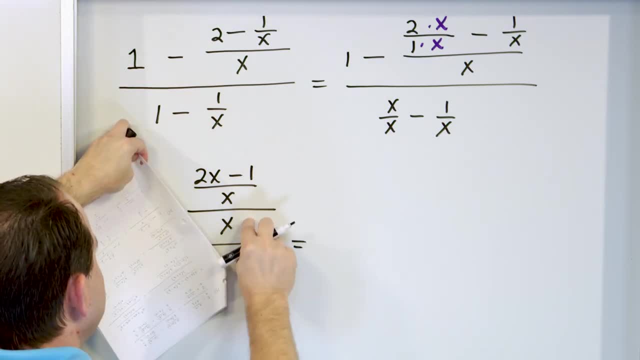 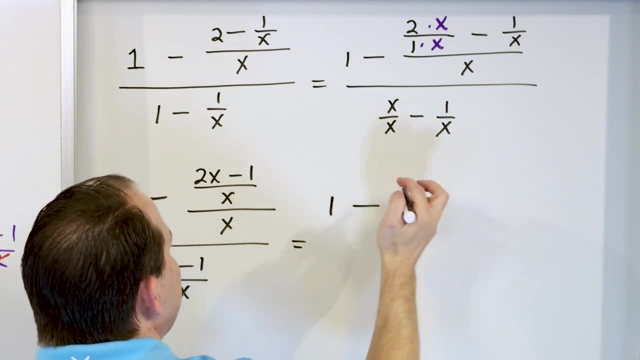 So here again, ignore this, ignore this. We have a fraction divided by a fraction. We have a fraction divided by a fraction. Of course it's just x, but we can think of it as x over 1.. So we say 1 minus. this guy will change to multiplication 2x minus 1 over x. 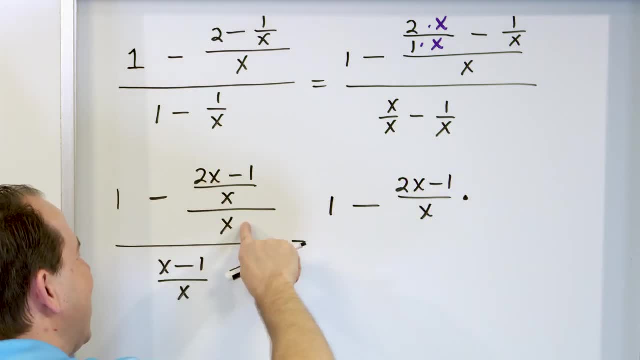 Change this to multiplication And then this x is really x over 1.. So when you flip it over, it becomes x over 1.. It becomes 1 over x. all right, Let me just double check myself. Yeah, 1 over x. 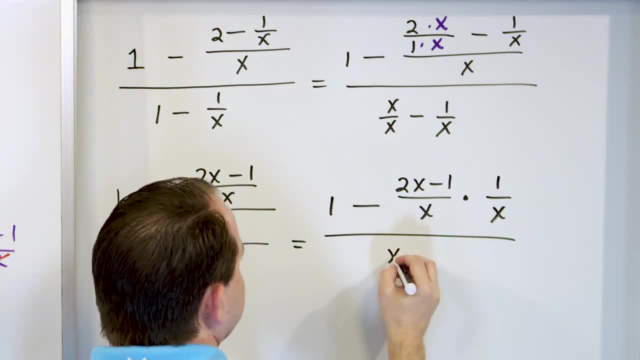 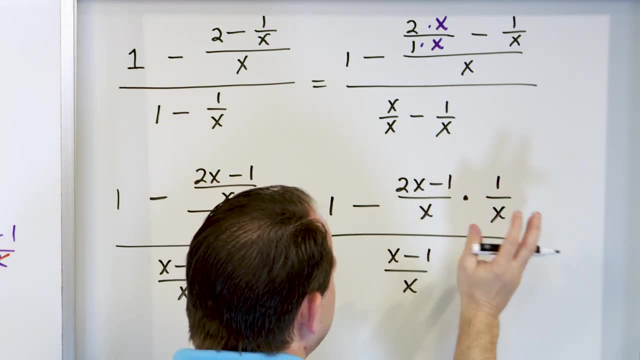 And then in the bottom, nothing we can do here. We're just going to leave it x minus 1 over x. So here we're at the point where we can multiply these fractions. We really can't cross-cancel anything, so we're just going to multiply it. 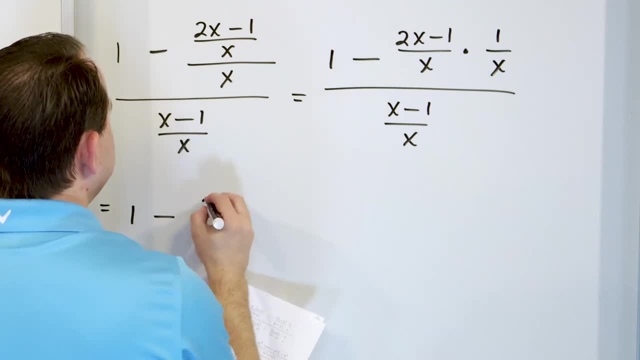 1 minus 2x minus 1 times 1 gives me 2x minus 1.. The bottom is: x times x gives you x squared. Now things are starting to look simpler: X minus 1 over x. Now I know this is still ugly, but it's not that bad. 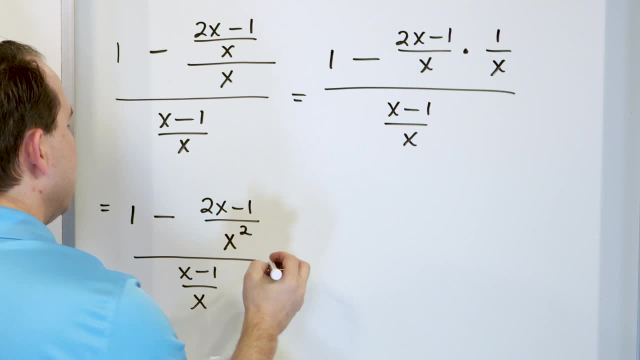 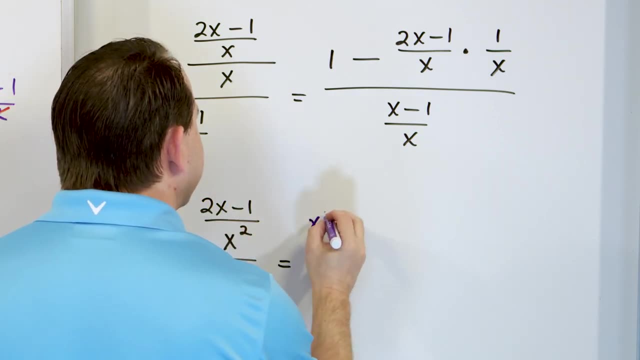 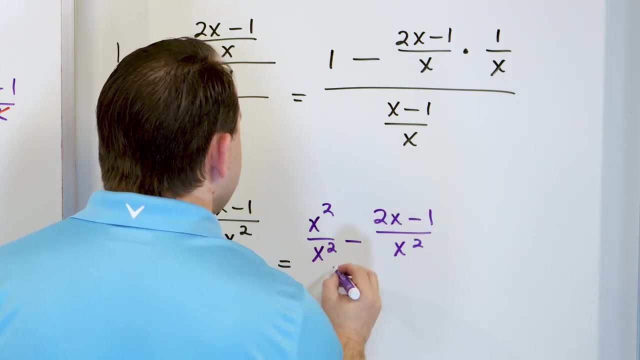 Now we have 1 minus this. We have to get a common denominator here. So the common denominator I'm going to shoot for- I'm going to switch colors here- is x squared. So I'm going to write this: 1 as x squared over x squared, minus 2x, minus 1 over x squared. 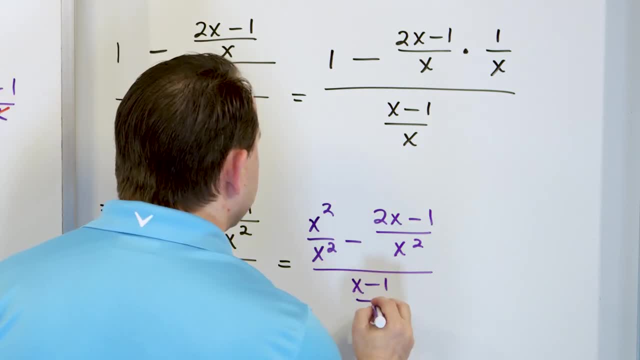 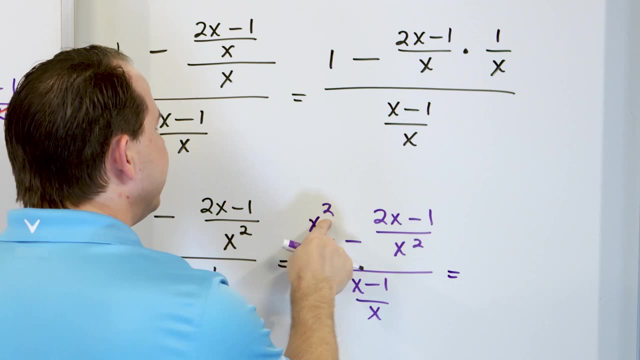 On the bottom. I'll leave this exactly where it is: x minus 1 over x. So then in the next step, common denominator, we have it. So it's this minus this. So be careful, because when you subtract it it's minus the whole quantity. 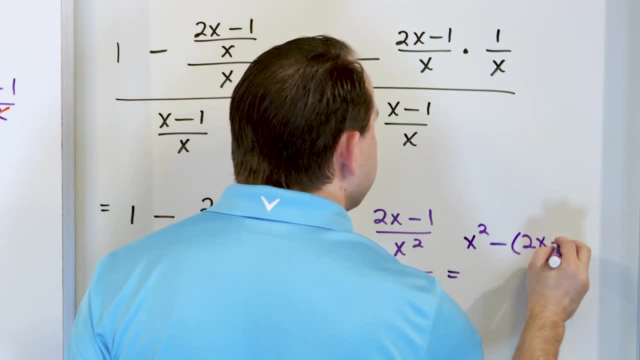 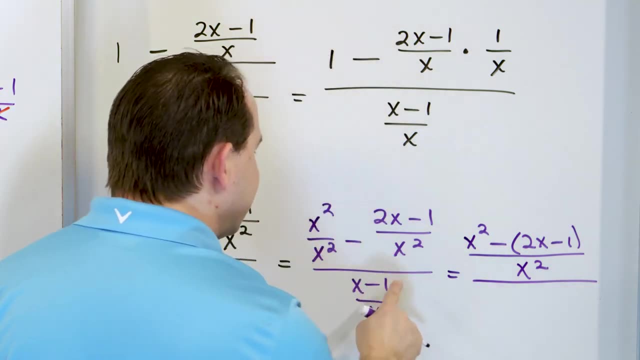 So you say x squared minus quantity, 2x minus 1.. You need to wrap that in parentheses. In parentheses to avoid any problems with signs. you have an x squared, Then down here you have an x minus 1 over x. 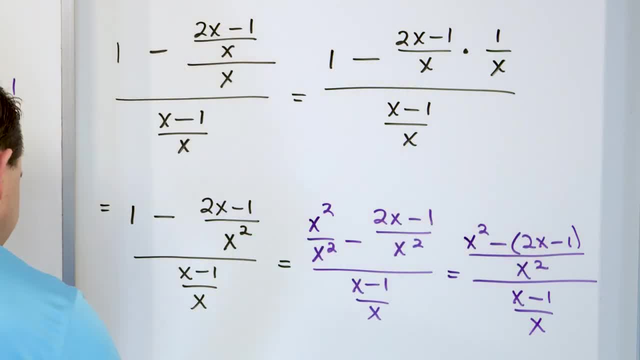 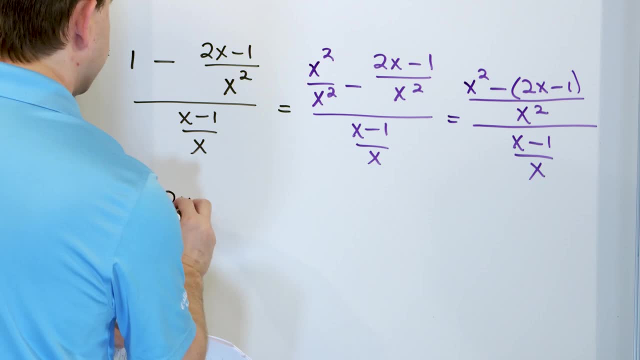 Now let's take a time and distribute the negative sign in. Let's switch back to black. So what we will have is x squared minus 2x plus 1.. It's minus 2x plus 1, right, And then here we have x squared. 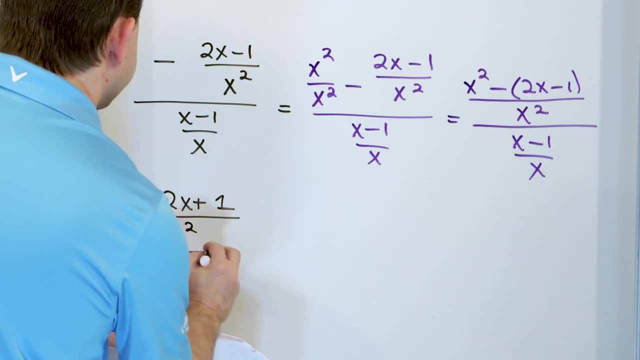 And then here we have x squared, And then here we have x squared, And then on the bottom of this guy we have x minus 1 over x. Now, at this point I think we can flip and multiply again, because we have a large fraction. 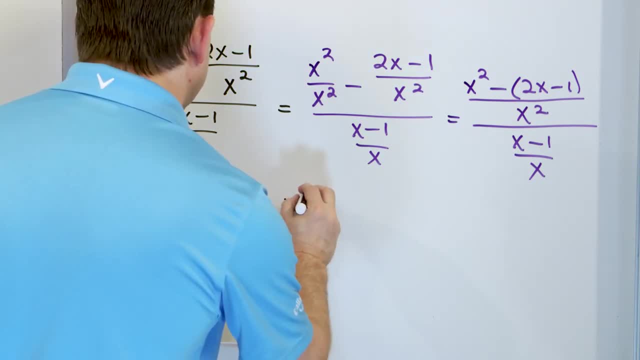 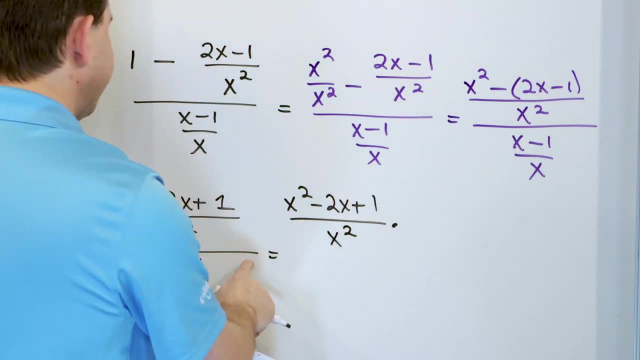 divided by a fraction. So it will be x squared minus 2x plus 1 over x squared. Change this division to multiplication, but we take the bottom fraction, flip it over x over x minus 1.. OK, Now we don't see anything obvious. 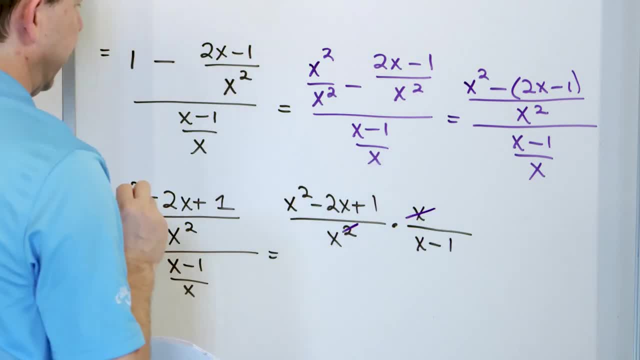 We can cancel here, But we do have a single x which can cancel with that single x, right? And then what we're going to do, what we could do is just we could say we're done right. We'd say this times, 1 is the numerator. 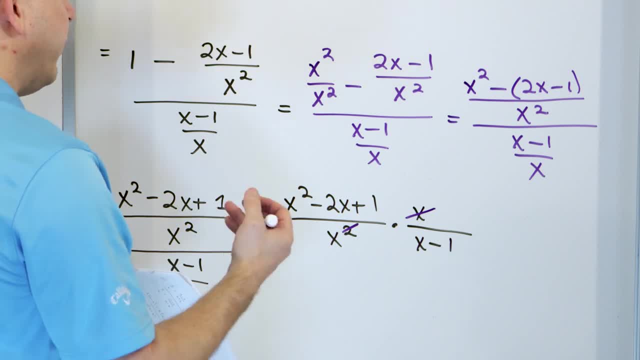 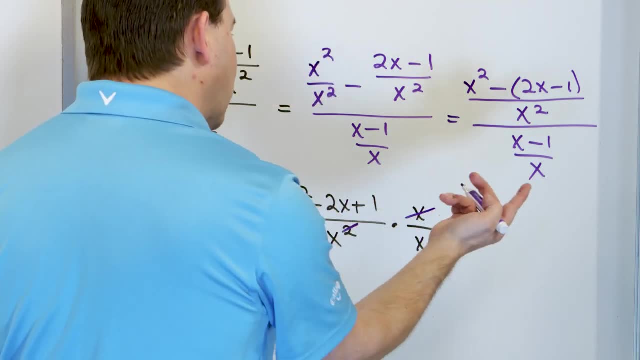 This times this is the denominator, But I've been telling you always try to factor things, And this looks like something ripe for factoring. So what do we have? It's going to be this times 1.. So the numerator is basically going to be: we're going to try to factor it. 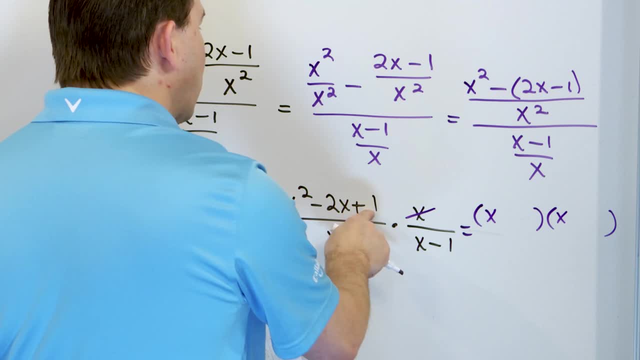 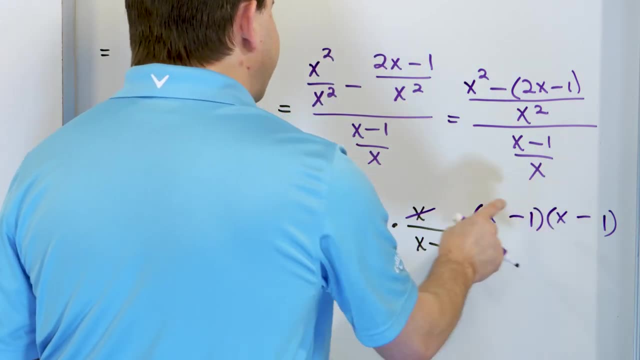 We have an x squared, So we have an x and an x, We have a 1. Which means 1 and a 1. And it's got to be a negative inside, So we have to have minus and minus. Double check yourself. 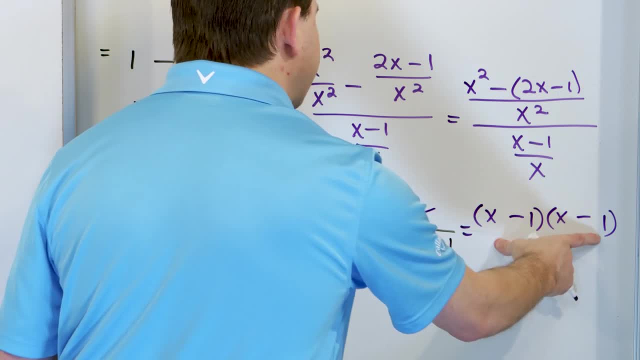 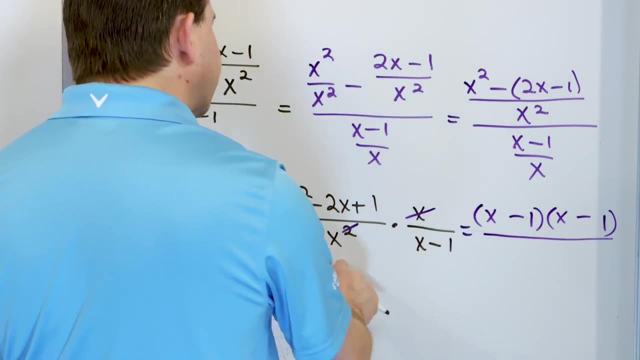 x times x is x squared. Inside term is minus x. Outside term is minus x, which adds to minus 2x. Last terms: multiply to give me positive 1.. On the bottom I've got these multiplied, which is x multiplied by x minus 1.. 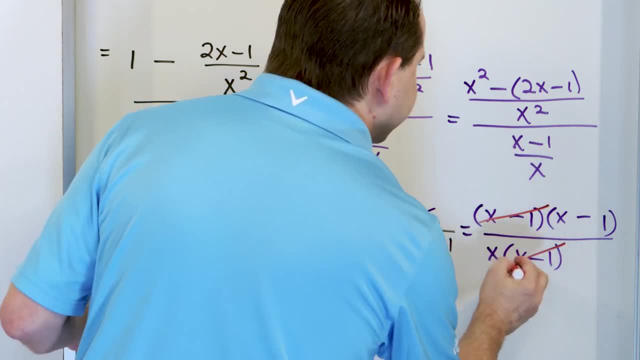 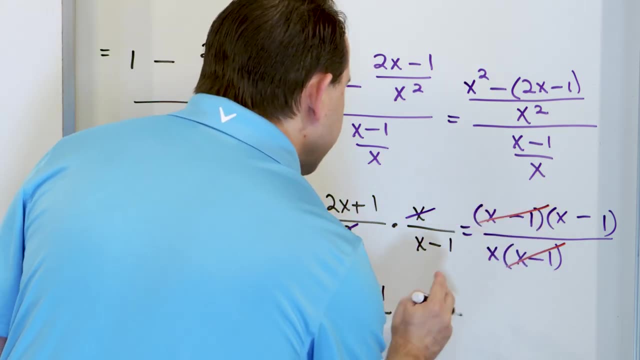 And you can see that the x minus 1 cancels this x minus 1.. So now we finally get it down, And I just have barely enough room. It's going to be x minus 1 on the top, only a single x on the bottom. 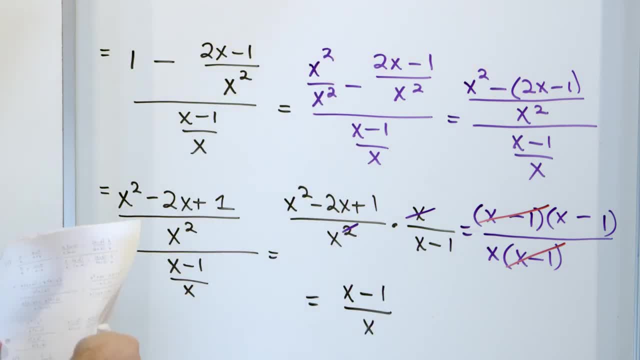 Double check x over. let's see here: Double check, Get my last page here. x minus 1 over x. That's the final answer. I always get a little nervous when we kind of do things without checking as I go, because 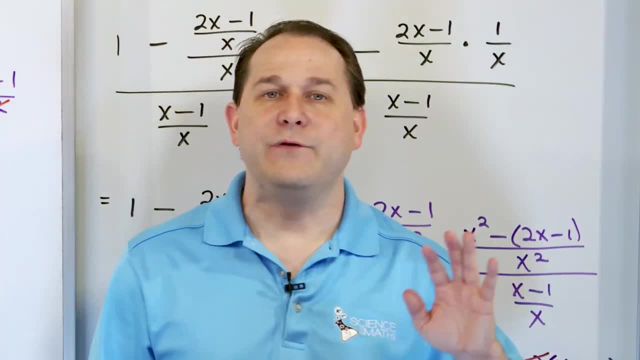 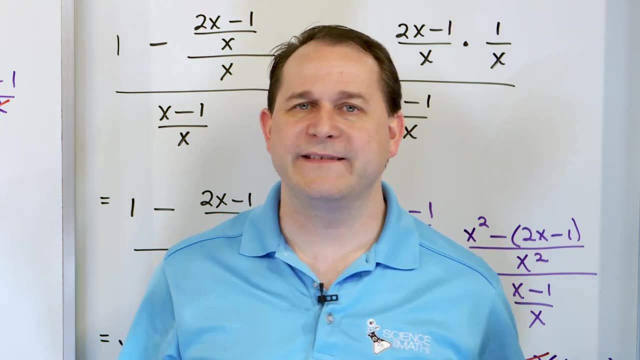 I make mistakes too. So, as I said, if you can do this problem, you can do any problem right, Because this was just gnarly right. But notice that it was incorporating all of the same skills, just lots and lots of nested. 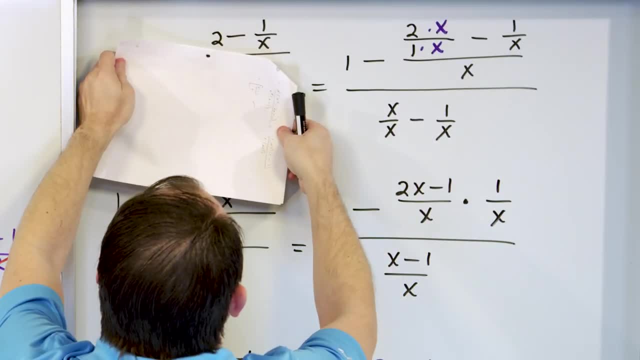 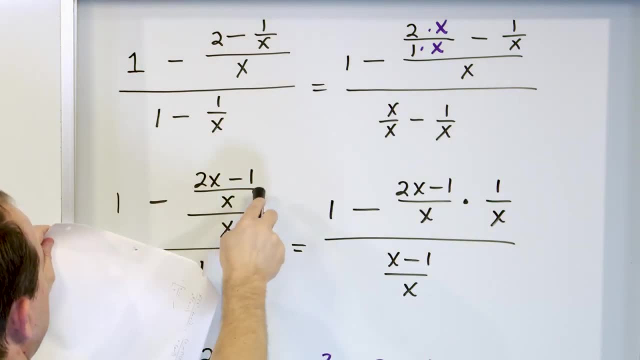 versions of them. You know how to find a common denominator between those fractions. We did them many, many times. So you have to do that over here right. And then you get down to where that's done right. Then you have fraction division.